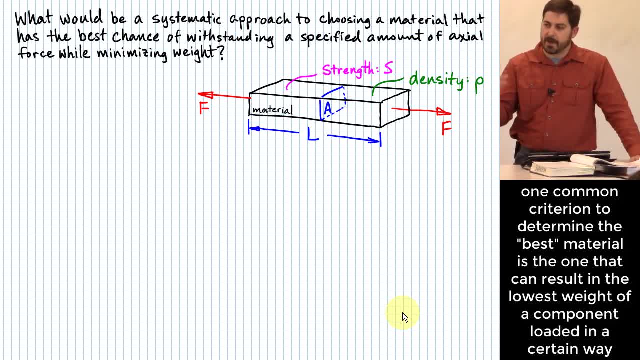 And when you're doing design, when you're doing mechanical design, the word better is always kind of, you know, contextually based. What do you mean by better, right? And so what I've put up here is one of the criteria that is sometimes used to try to. 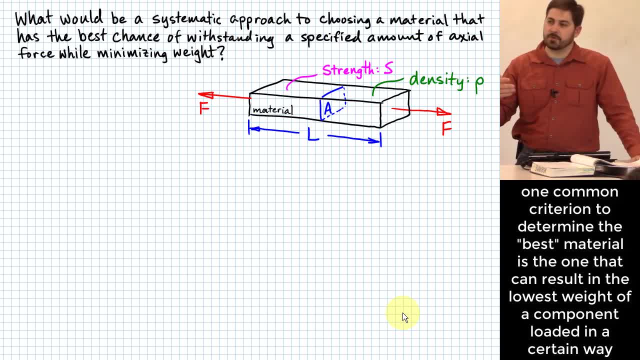 determine a material that might be the best or kind of a design that might be the best. One of the really common ways of doing that is to try to figure out what's going to reduce weight right. Reducing weight does a couple of things. 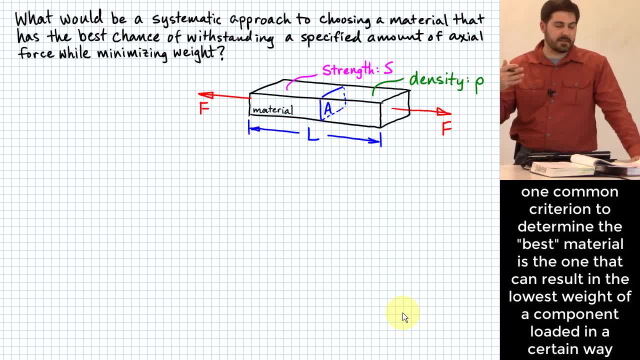 One. you do use less material, right, You have less of it to have to have to. You have in there, And then a lot of the designs that you make might actually be things that need to move. And any time you can reduce weight, it is that much less energy that it takes to start. 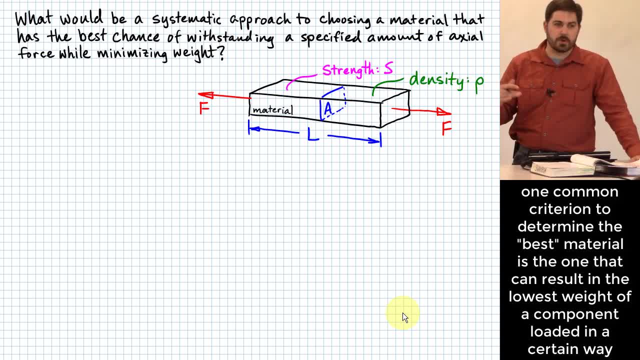 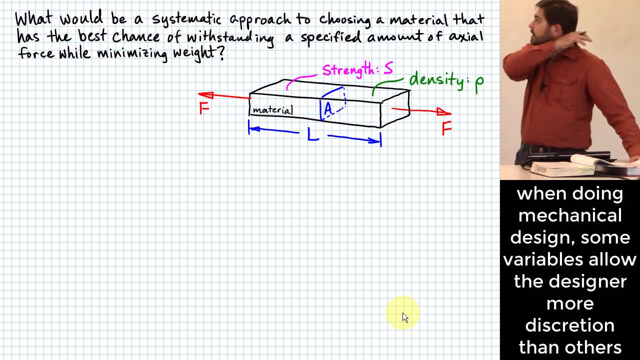 and stop things moving and that kind of stuff. So reducing weight is one of those things that's very often something that we need to try to think about designing around. So what I'm asking up here in this question is what would be a systematic approach to. 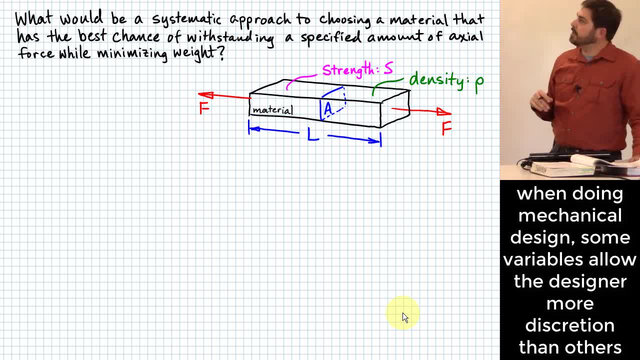 choosing a material for an application like this that has the best chance of withstanding understanding a specified amount of axial force- that's the F, right there- while minimizing the weight, okay. So let's think about things that if that was an actual member that had to be doing a particular 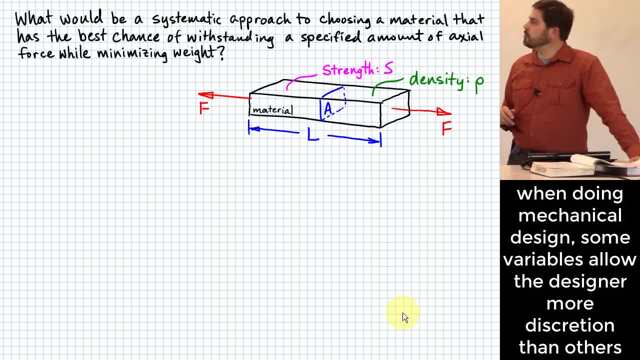 job in a machine. let's say: what are some things that you are more likely to be able to control in your design, or things you're less likely to be able to control? right, Because whenever you're doing design, what you're doing is you're trying to make decisions. 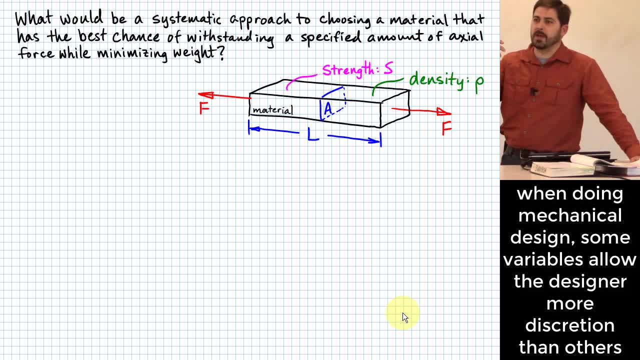 as to you know, maybe, what kind of material you're going to use, Right, And you're trying to settle all that up to where it's the best situation that you can have, And this is saying what would be our best. you know what would be a strategy about trying. 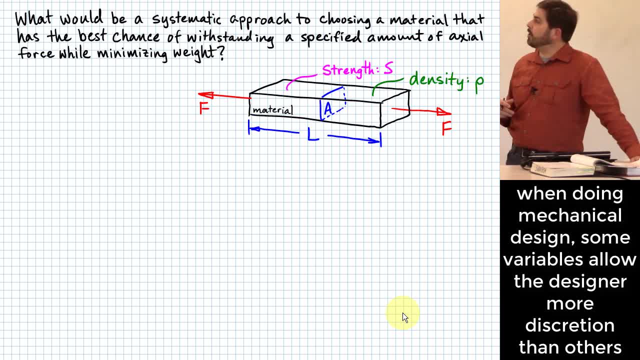 to find the best material to be able to minimize weight while still carrying the load- The things that we'd probably be able to control right. well, let's think about the things we couldn't control, maybe first. One of them is how much force we have to put in the machine. 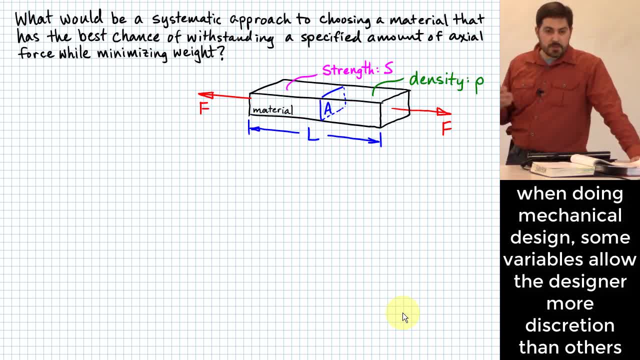 So a lot of times we're talking about a lot of things that we're trying to control. One of them is how much force it needs to be able to carry Right The way. the problem- at least the way the problem is stated- is basically, you need to. 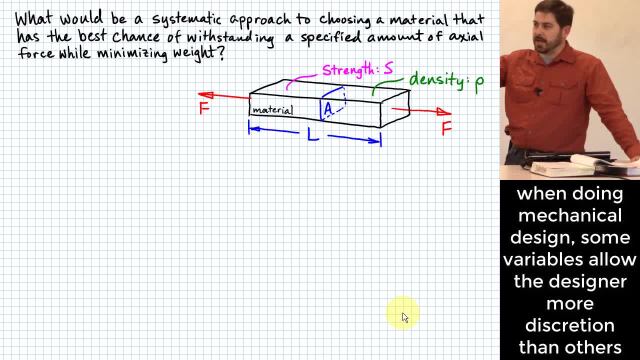 be able to carry a specified amount of force, right, So it's no use complaining about that force being too much. right, Because that's the job and we've got to get that done. right, So we're not. let's say that force is one of the things that we're not going to say. 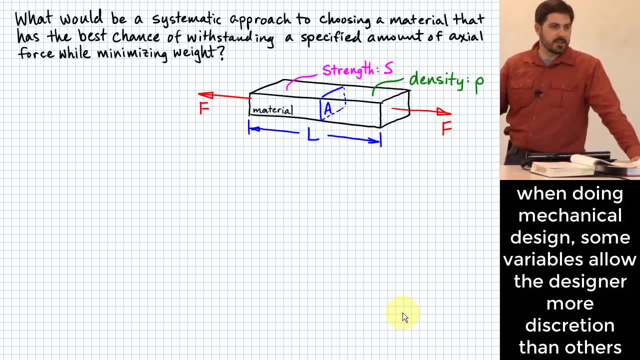 that we're free to change what that number is. okay. What's another thing that we might not be free to change? Yeah, I mean, you're thinking very, very broad. He says budget: right, You might not be able to change your budget. 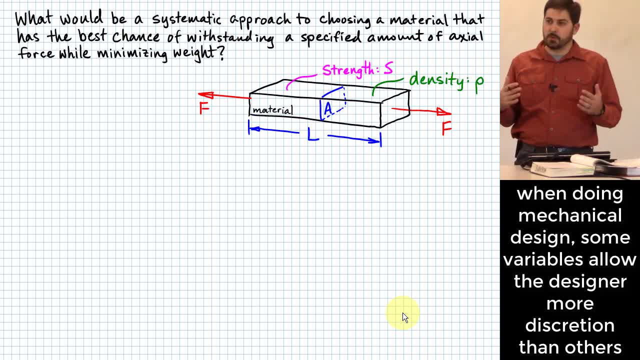 Although what you'll find is that if a job really needs to get done in the world, right, it really kind of ends up not mattering very much how much it costs, Like if it's something that actually does need to be done, and especially the larger. 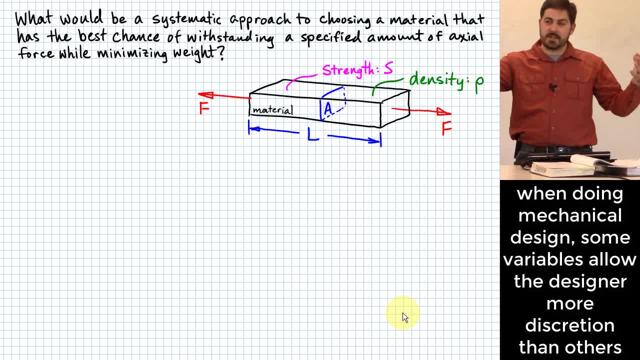 number of people it affects. if it doesn't get done, then you end up seeing that society will figure out a way to pony up the money to be able to get done whatever needs to get done, right? So good, good, That's a good thought that you had there. 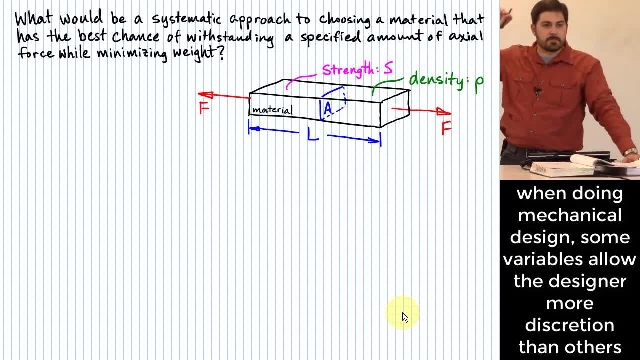 But in terms of the variables that are on this figure, right, what's something else that maybe in a lot of cases, you wouldn't be able to control? about this example: Okay, I actually. he says cross-sectional area. I would actually say that's probably the one you're most likely to be able to control. 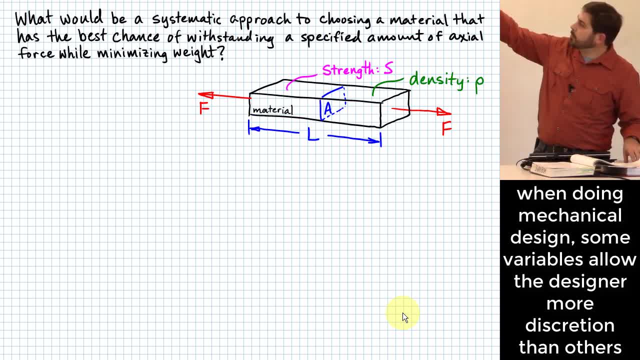 right, Because if you think about this, what you're trying to do, maybe with a member like this, is transmit force from one place to another, And it's likely that you might have some other parameter in your, some other consideration. I should say in your design that you're trying to do that would specify how long this little 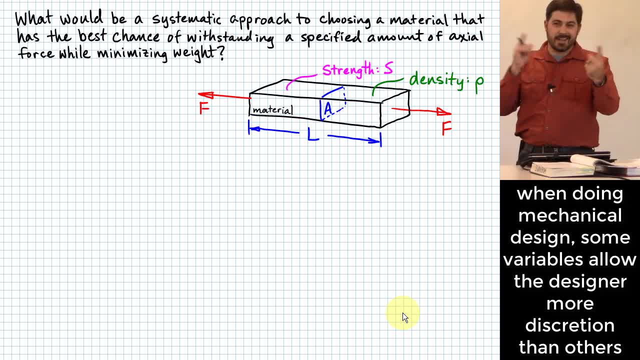 force transmission link might need to be right, So it's that's another one that might not be so easy for you to control. On the other hand, cross-sectional area is more likely to be one of those things that you could say: well, whatever material I've got, I can let that cross-sectional area get. 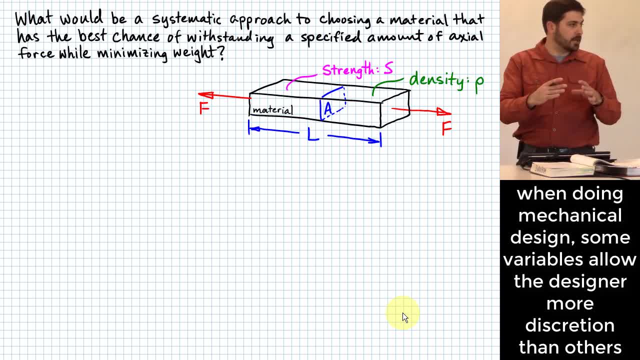 however big it needs to be in order to be able to carry it. So it's, that's another one that might not be so easy for you to control, Right. So there are some things, and you know we're kind of talking about some hypotheticals here. 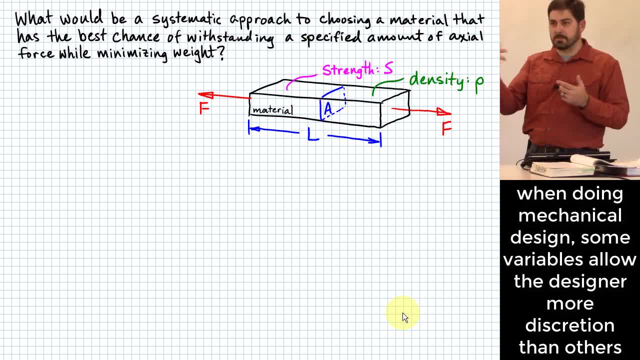 but I'm trying to get you to think through. in any design there's usually some things you can control and there's some things you can't control And you have to try to most beneficially pick the things you can control to make something that works. 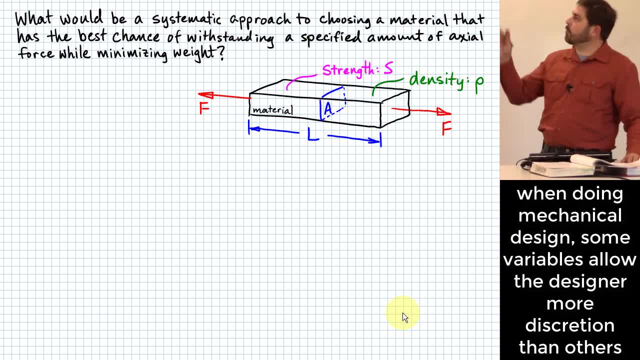 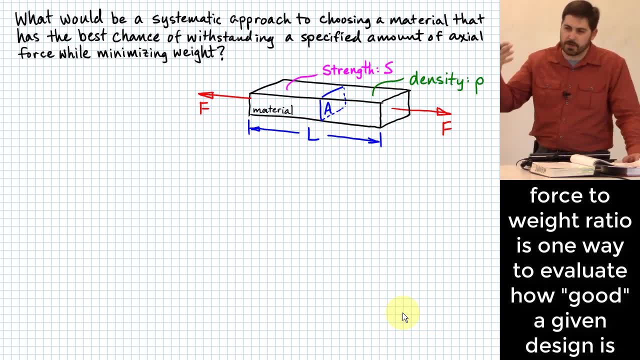 Right. So if that's what we're dealing with here, and what we're trying to do is minimize the weight while still being able to carry the load, What's one way we can sort of construct in our mind when we've come up with that you? 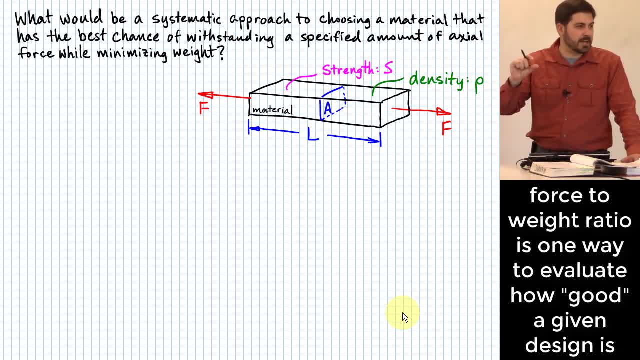 know, like a number. maybe that allows us to score whether we've got something better or worse. with respect to that question, Could you do like a ratio? What do you think? Maybe, Okay, Let's think about maybe a ratio of How much force it can carry per how much it weighs. 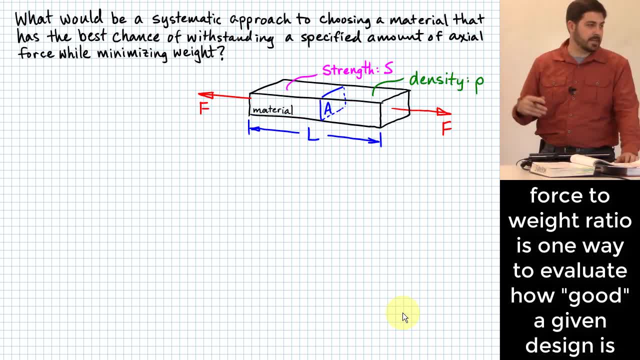 Maybe a ratio like that might be a good way to score how good this thing is at doing what it's doing Right. That way, the more it weighs, the lower the score ends up being Right. So let's think about having something like that where we basically say: you know, we're. 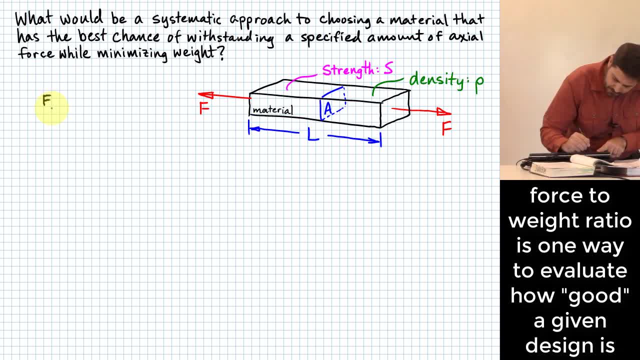 going to try to take this ratio of F over W, Where F is the force and W is the weight, And what are we going to try to do with that ratio in order to come up with the best thing we can. You want to try to get this thing larger or smaller. 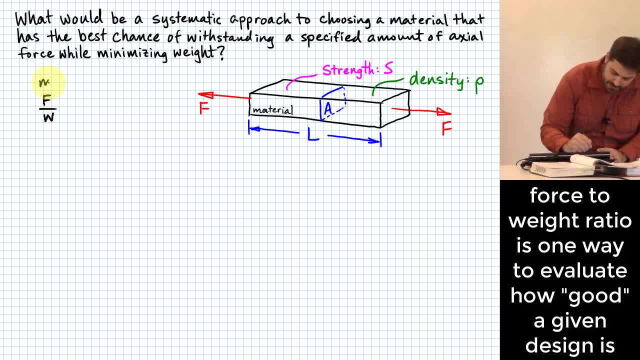 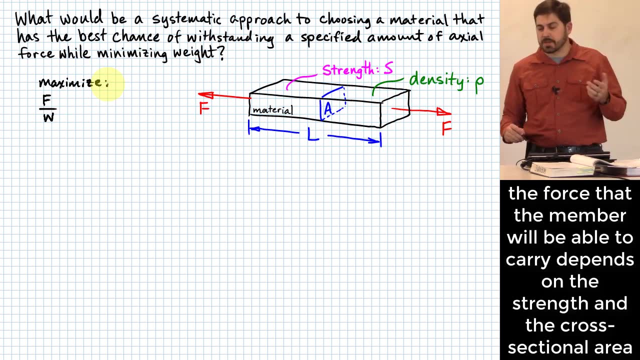 Larger, Larger. Okay, So you're going to try to maximize that ratio? Okay, Well, let's think about what composes these ratios. What controls how much force can be applied to this body before it can carry the load? Okay, 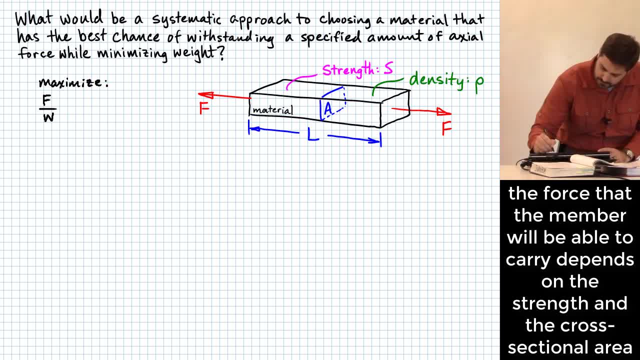 Let's say it fails. Okay, We basically for an axial load like this. the stress in it is going to be equal to force over area, Right? Well, how much stress can it carry? Okay, Depends on the material, And one of the things you see up there is that I've indicated some things about this. 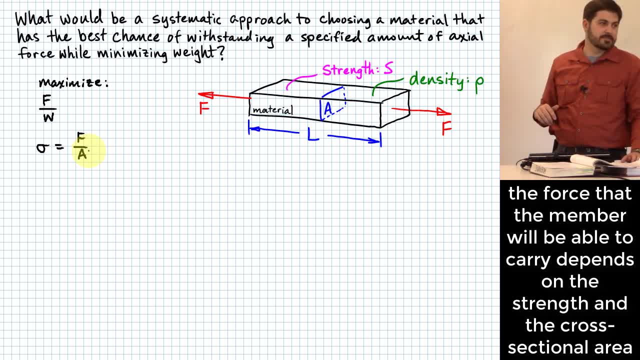 material. Let's say the material has a strength of S Right, And I'm trying to keep this very general. I'm not saying this is a yield strength or an ultimate strength or necessarily any specific kind of strength. This is essentially the stress that causes it not to function anymore. 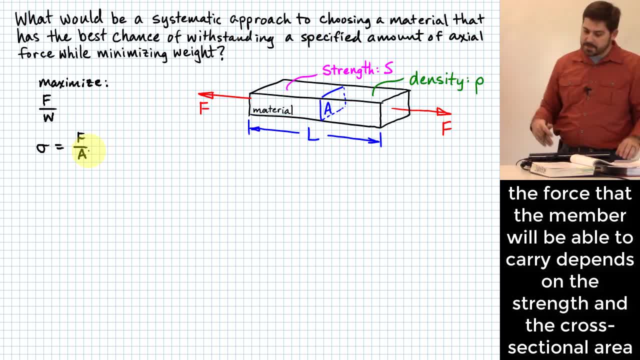 Right, And we call that a strength. Okay, So let's say that it loses its function once the stress level gets up to that strength. Right, And so what we can say here, then, is that this can be rearranged as: F is equal to S. 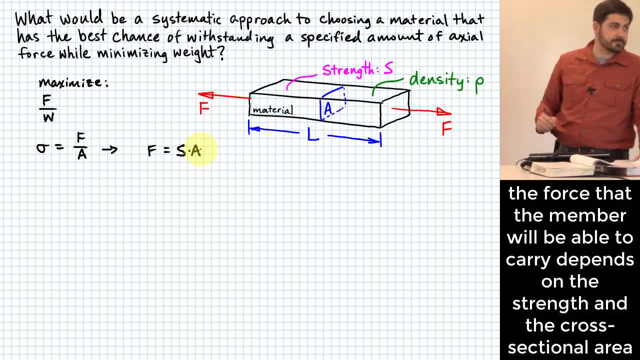 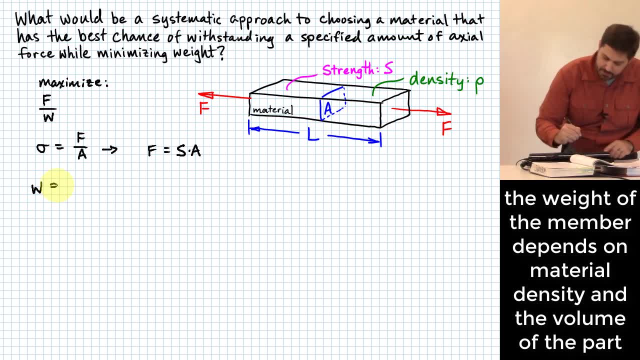 times A, Right. Okay. What about W? W is the weight. How would I calculate W for a body like this? Okay, You have density times. the area Right. Times the length- Right, That's how much this little thing is going to weigh. 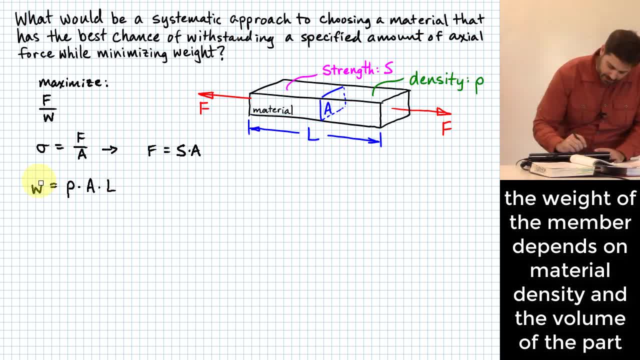 It's the volume times the density And really I think you know we can think of that. I'll leave it as W there. Technically it would be a mass Right If I'm using a density Close enough. 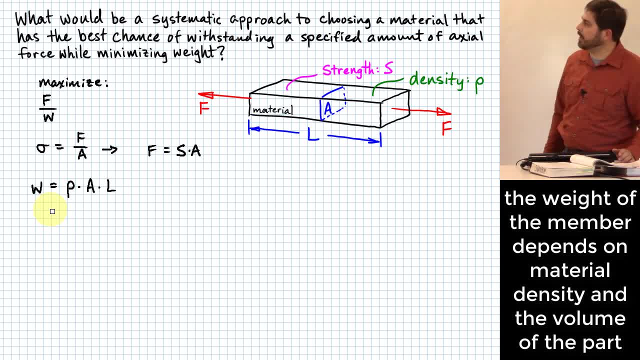 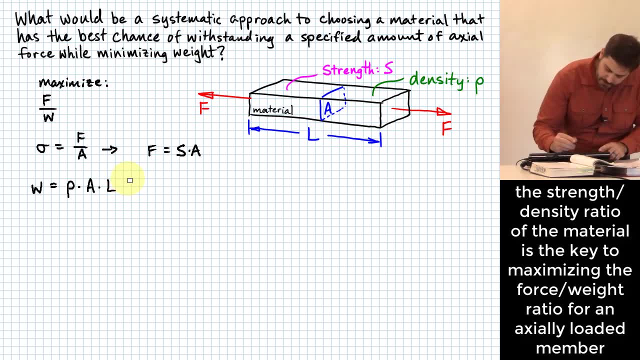 Right, We'll kind of think of mass or weight Either way, Okay. Well, what now if I take these? you know these two things, This piece right here and this piece right here, Right, And I go ahead and do and I kind of score this fraction. 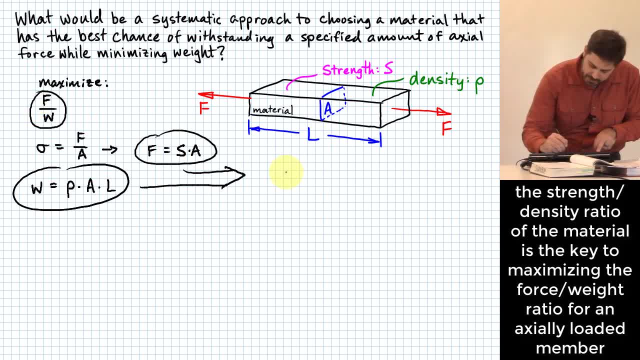 Right, So I end up with S times A over rho times A times L. Okay, What is this going to give you? Okay, This is basically that F over W. It's going to be equal to this. Can that be simplified at all? 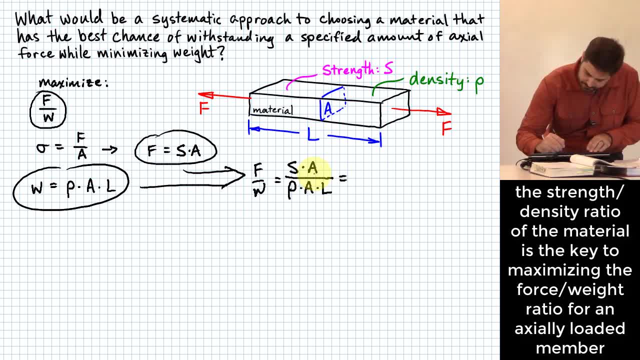 Okay, The A's cancel, Okay, Right, And we're left with S over rho, L, Right? So basically, and let me do this, I'm going to group S and rho together, Okay, And then multiply by L. What's the difference between variables like S and rho and a variable? 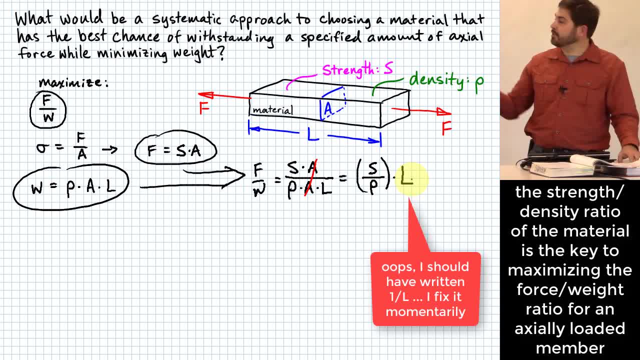 like L, Okay, The length is. that's something that specifies the size of this thing, the geometry of this thing. Okay, So what are the properties of this thing? S and rho, What are those? Those are material properties. 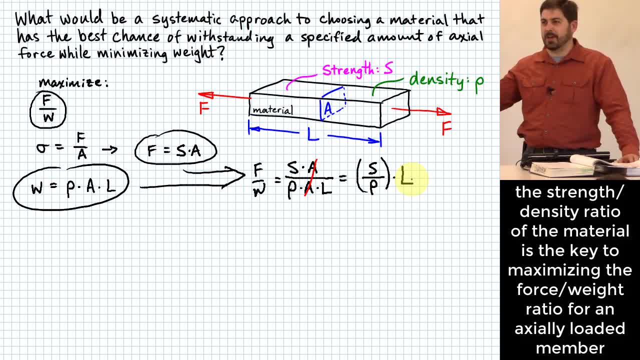 S and rho are things we can't pick anything that we want Right. S and rho are things that we have to choose, a real material that will have a particular strength and a particular density to it, And there are only discrete choices that are out there for those values, depending on what. 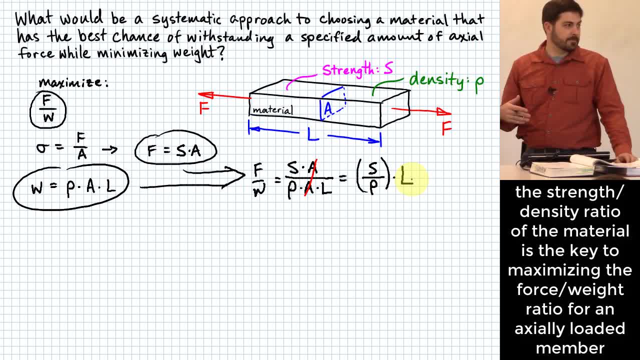 kind of actual materials we might be able to use, Okay. So here's where I'm going with this: L is not something that we would be able to compute, Okay, L is something that we would be able to control, And so it's going to be what it's going to be. 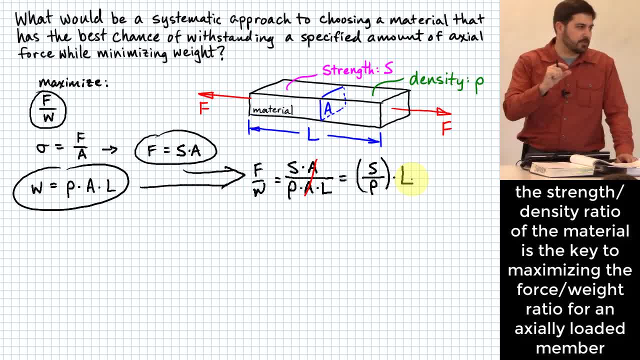 S over rho then becomes this kind of scoring factor for us to know whether or not we've got a better material or a worse material to be able to do this job. Okay, I know, this is kind of a different way to think because we're not doing an actual problem. 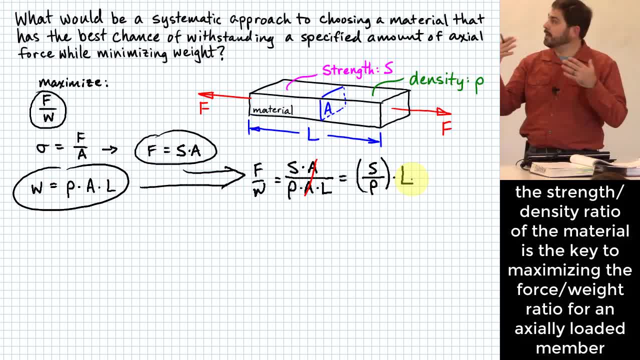 with real numbers. I'm trying to get us to think about the concept of how would you end up scoring individual kinds of material to know whether it's better or worse than another for being able to carry a load like this? Yeah, Shouldn't that L be 1 over L? 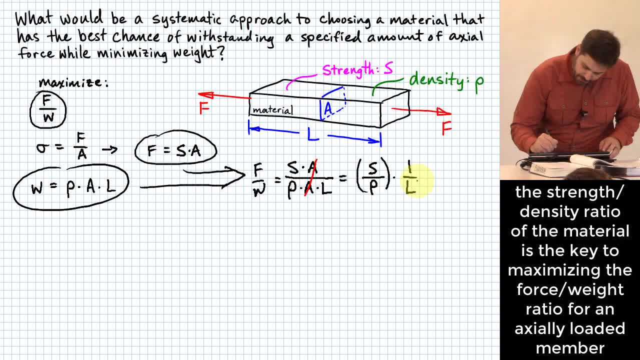 Yep, Sure should be. Thank you. She said: shouldn't that be 1 over L? And it should be. I just wrote it wrong. Okay, But it doesn't matter anyway. Right It's. that's not the focus of what we're trying to do, because the length is going to have. 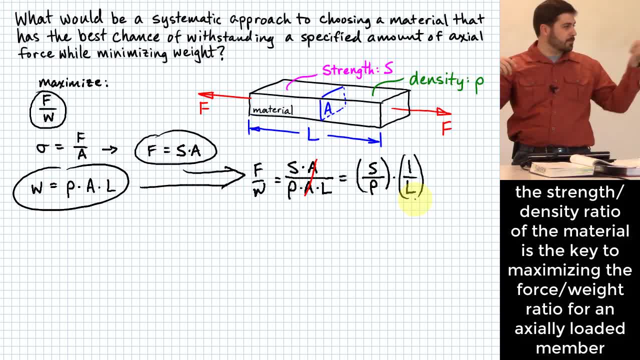 to be what the length is going to have to be, and it's going to be the same whether you're building a part out of aluminum or a part out of steel or a part out of wood, Right? So, Um, So what we're trying to do here is that there's a particular factor that we can look at that. 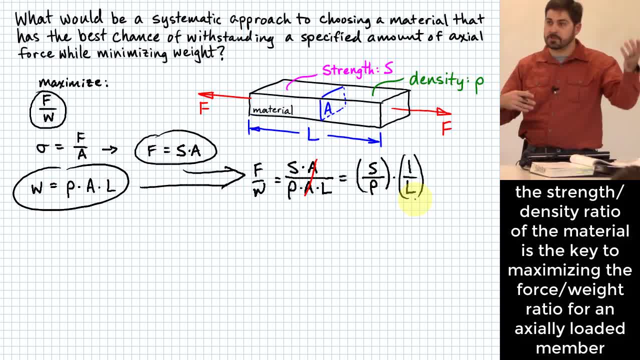 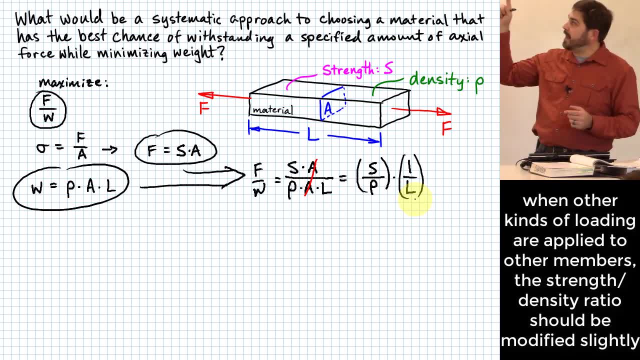 will allow us to score materials and know whether they are better or worse at carrying this kind of load than another one. Okay, Now, this is an axial load. I specifically did this particular problem for an axial load. Do you think it ends up being the same for a load like a flexural load? 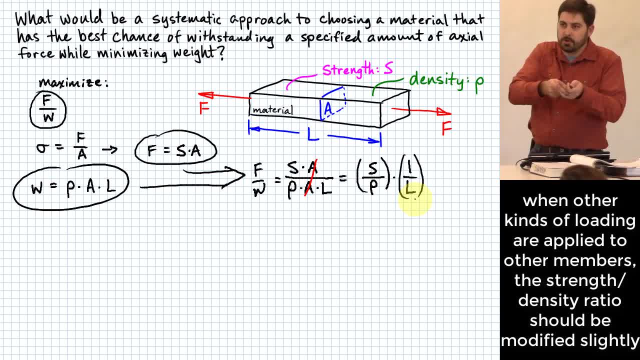 In other words, if you pull something straight down its axis or push down, you know, actually pushing is even a little bit different, Right, Because you have the possibility of buckling, Right. But let's say you're pulling along an axis. 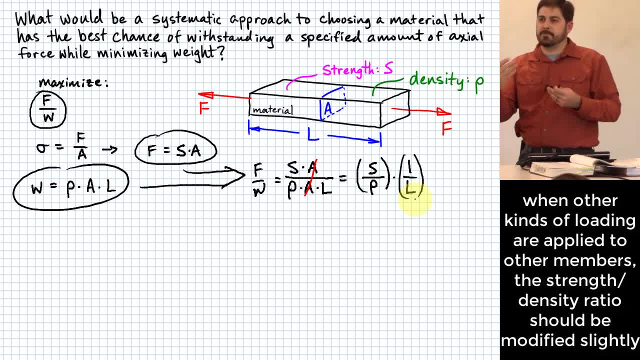 Are you going to end up with the same factor here, do you think, as if you have a case where you're trying to flex it? Okay, I'll go ahead and tell you. no, it will not be the same, but it will be in the same form. 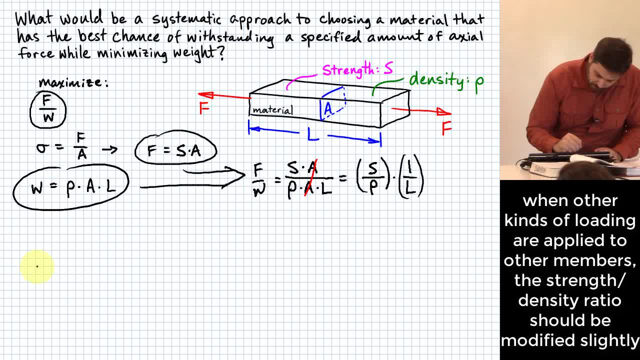 Okay. So I'm going to say down here for flexural, and actually it's the same for flexural and torsional, Okay, Okay. So in the same format, it's just: instead of just S over rho, we have S, okay, and this: 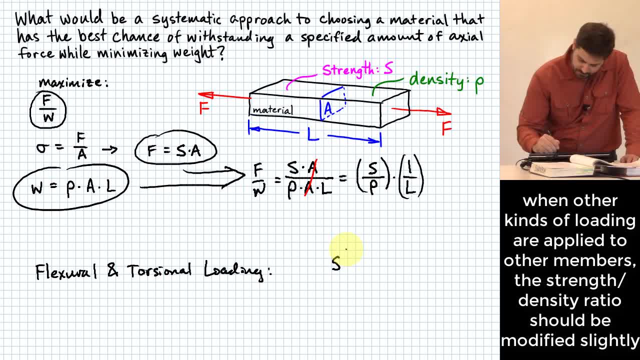 is going to be a little bit weird, but it's S to the two-thirds over rho. okay, And if you want to see how they come about, you know coming up with that number. they actually do that in the textbook. That's why I didn't show you that one, because they have that worked out in the textbook. 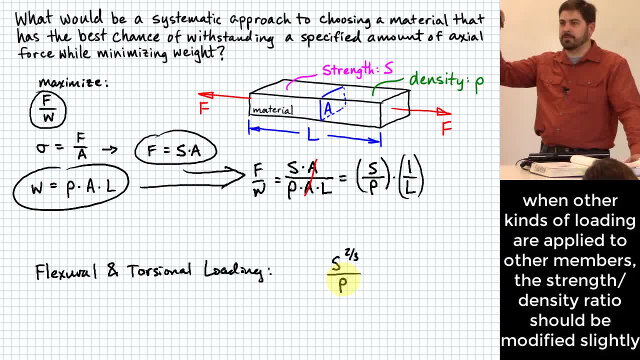 how they come up with this factor of two-thirds. Okay, Well, why do we care about this? Let me show you why. It turns out that materials, once you've chosen a material family, they tend to cluster together to where these ratios of either S over rho or S to the two-thirds over rho. 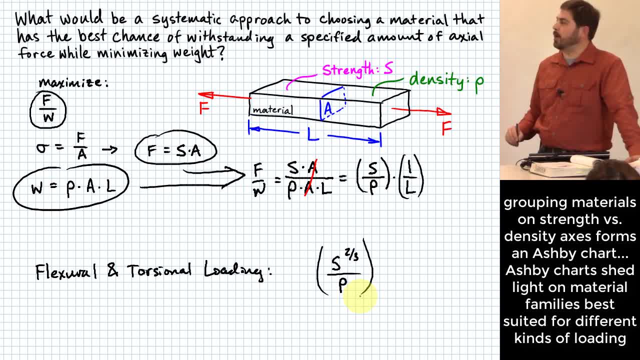 they tend to sort of cluster in these particular kind of regions, and then that lets you decide what you think might be the best you know ratio for each of the two-thirds over rho. Okay, So I'm going to go ahead and show you how that works. 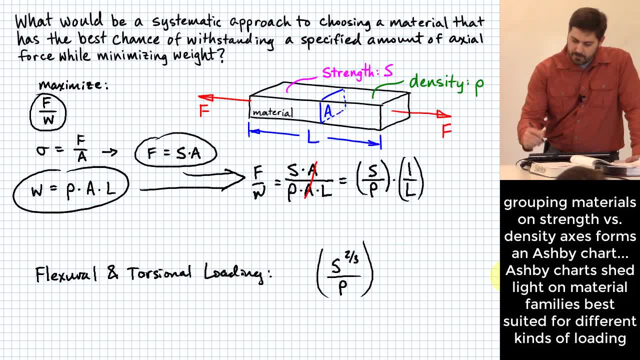 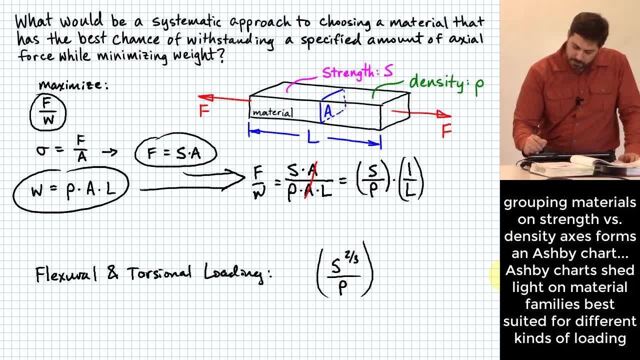 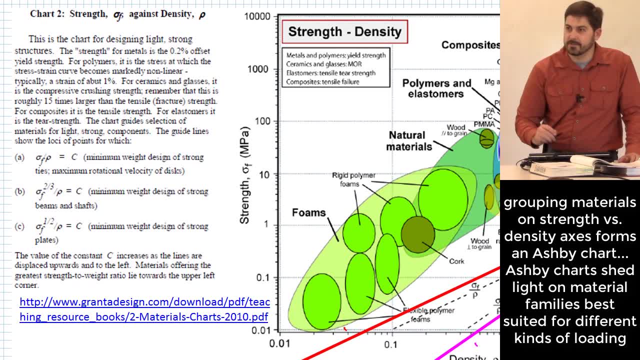 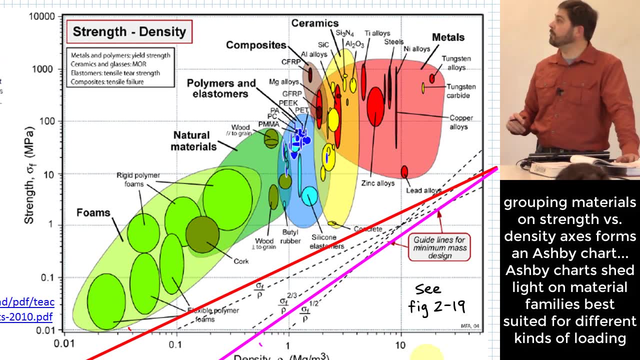 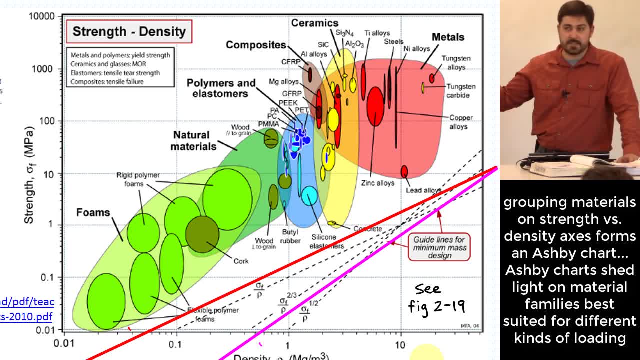 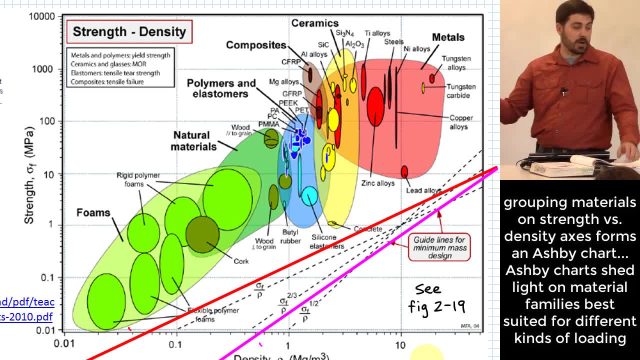 Okay, Okay, that increasing the area won't cost you too much in terms of the weight. Does that make sense? So this right here allows you to cluster these little groups of materials together and determine which ones might be better than another one. How do you do that? Well, let me show you this. 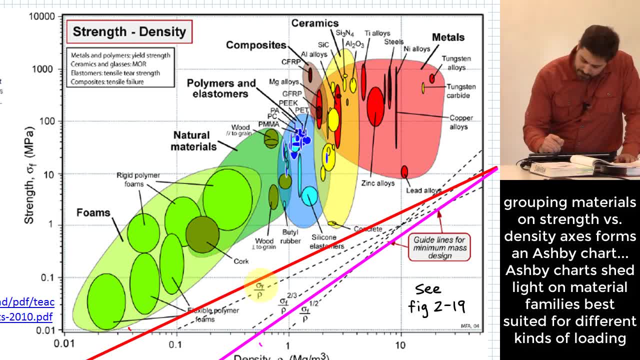 They have these little guidelines right here. You might notice, right here we've got sigma f over rho. What that means is if I'm trying to compare two types of materials with their appropriateness for being able to carry an axial load, and I want to know which one's going to be able to be a lighter candidate for a job like that. 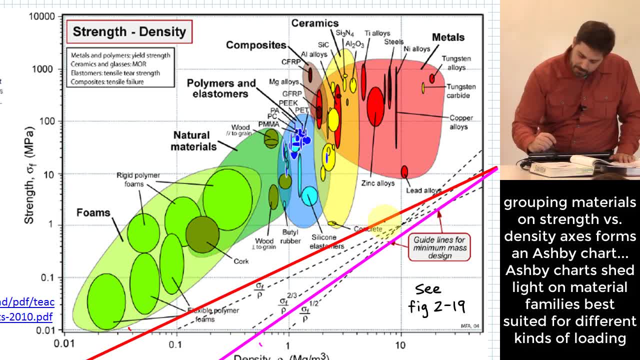 I can look at this guideline right here and think about moving it up. staying parallel to what it is right now- That wasn't a good color for that. Keeping it parallel to the way it is right now, but moving it up Right And. 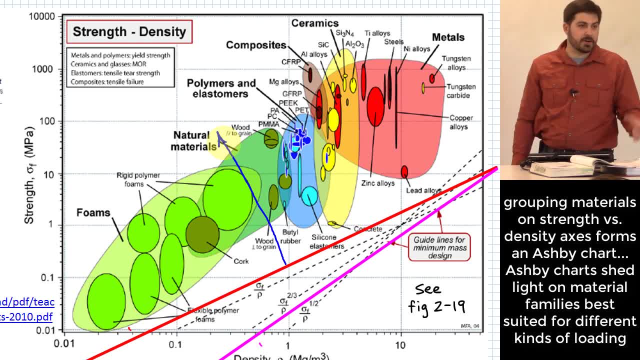 the things that are furthest out that direction, that I'm showing that arrow, are the best representatives on this little chart for things that would be good at carrying that kind of axial load. Does that make sense? So I've got this ratio and the more I can increase that ratio of sigma f over rho. 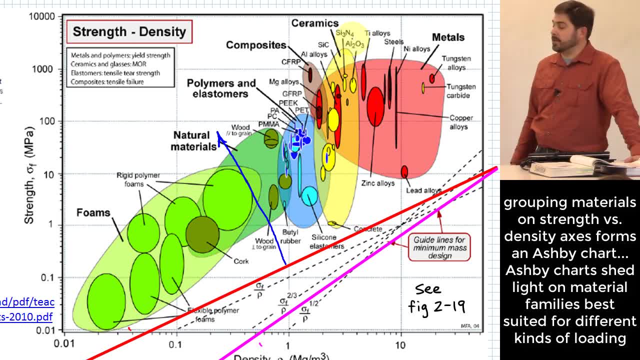 the more I can move further out and end up with a material that might be better at being stronger and lighter at the same time. Okay, So, like on this chart, what are some really good candidates then for axial loading? you know, to be strong and light at the same time. 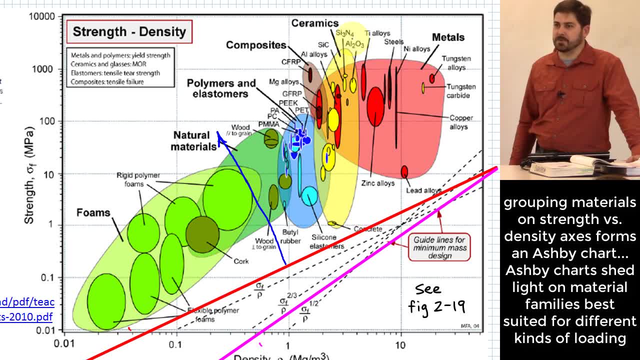 You see any that might be interesting ones that would stand out. Okay, Think about moving that red line up the direction of the blue arrow Right. What's the last thing that my red line would touch on its way out, on its way up that direction of the blue arrow? 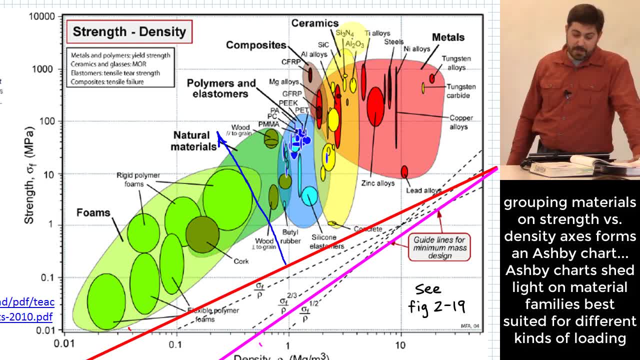 Maybe something in the composites. What's that? CFRP? That's carbon fiber, reinforced polymer. Right, And that's one of the reasons you see a lot of things made out of carbon fiber. It ends up being a pretty strong and light type of material. 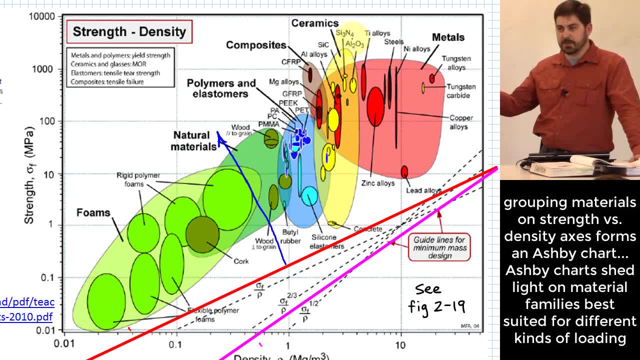 that can be used to carry certain kinds of loading Right. So I'm going to do an example here in just a minute. We won't necessarily dig deep into this chart right here, this second, but I wanted you to see that there's a big difference between a carbon fiber reinforced polymer. 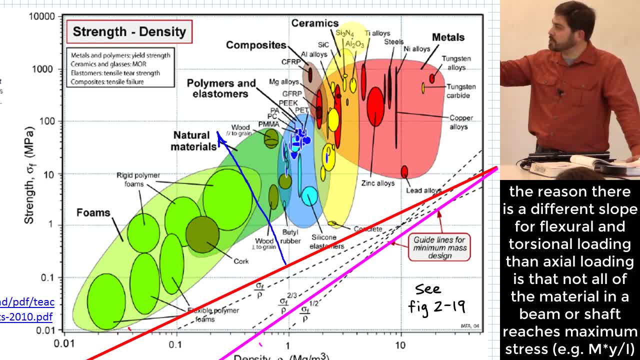 and a flexural or torsional loading, And you can see that there's a basis as to how they came up with the direction of these guidelines that they have down on the bottom portion of the chart And it's going to be different if you're talking about axial loading versus flexural or torsional loading. 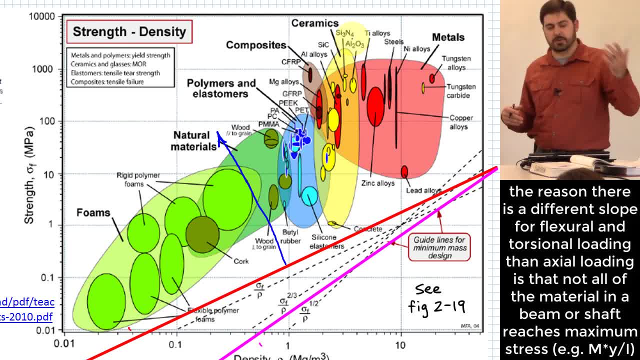 Let me talk about that for just a second. Why do you think it is different between axial loading and flexural or torsional loading? Why do you think there's a difference there? Say that again one more time. It is based on the kinds of stresses that are created within a member that's loaded in one of those directions. 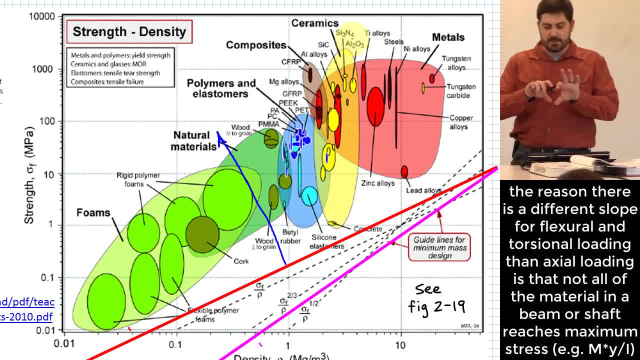 Let me ask you this. Let's say you just have a rectangular bar that you start to bend. Does all the material in that bar reach failure stresses at the same time? Why not? You might remember the formula that we had for flexural stress. 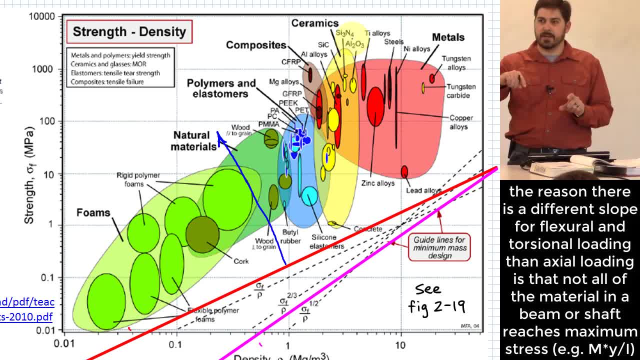 One of the formulas we had was my over i. And what was y? Yeah well, y is actually the distance away from the neutral axis, right? So if you go further out in the material away from the neutral axis, the more stress you're going to see. 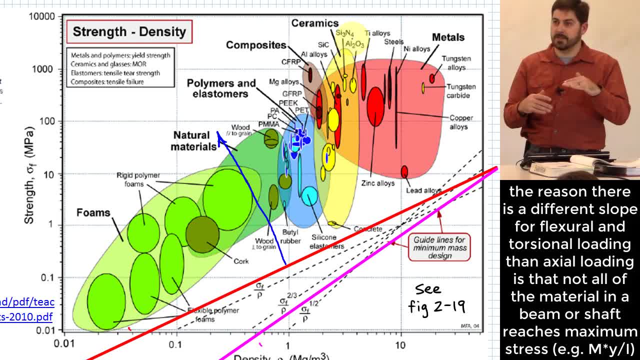 which means the material closer to the neutral axis is going to have lower stress. But the material closer to the neutral axis is still material right. It still weighs the same amount, Even though you're under utilizing its strength. Does that make sense? 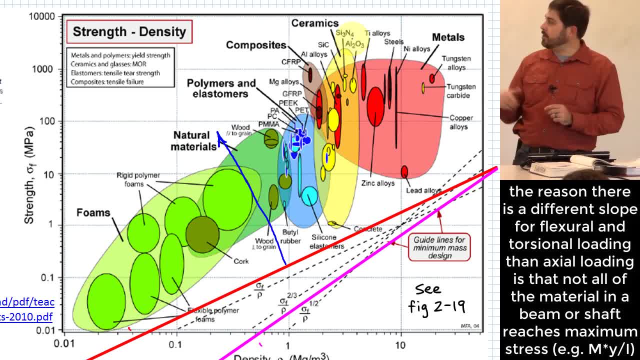 So that's the reason why the number for the- you know that you know- sigma f over to the two-thirds. that's why that exponent right there is different, because you're using that material differently, right? Same kind of thing with the torsional loading, right. 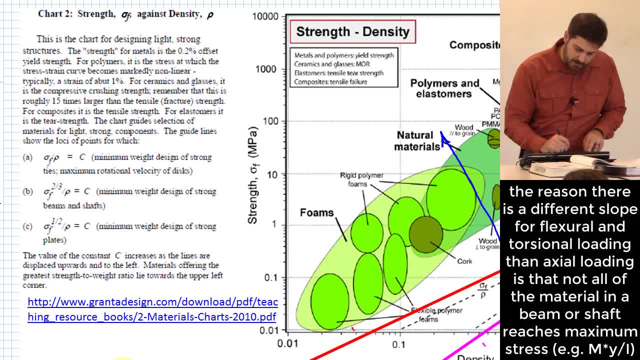 And actually, if you want to see you know a little bit of notes about this. it says here: you use this setup right here if you're trying to do minimum weight, design of strong beams and shafts or the one we just came up with. 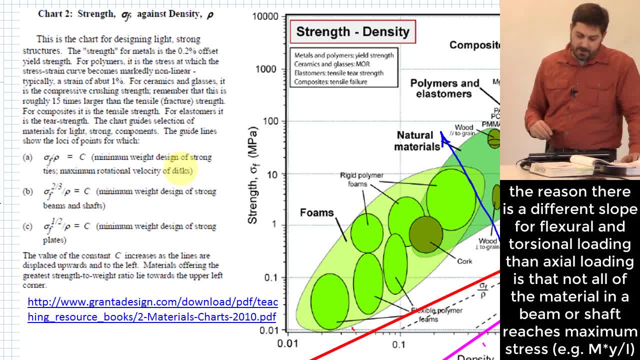 It says minimum weight, design of strong ties or velocity of disks. We haven't gotten into that yet, But when I first read this I thought that was kind of interesting. I don't typically call these two force members ties, but I looked it up. 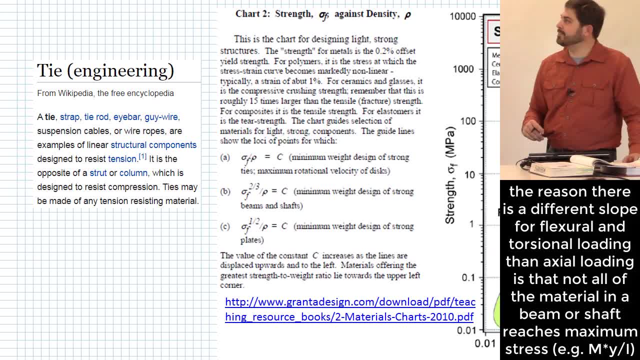 Wikipedia says that's a thing All right. So it says: in engineering you call this a tie, A thing that is a strap, a tie, rod, eye, bar, guy, wire, such and such and such designed to resist tension. Okay. 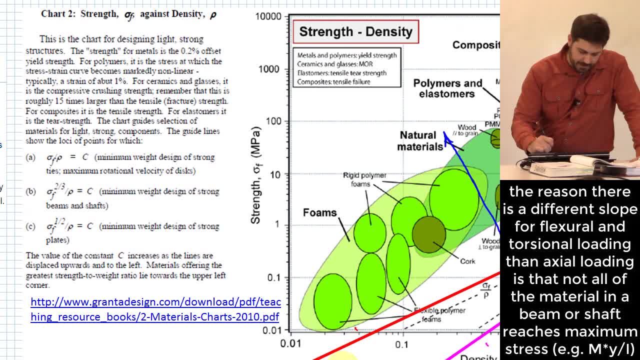 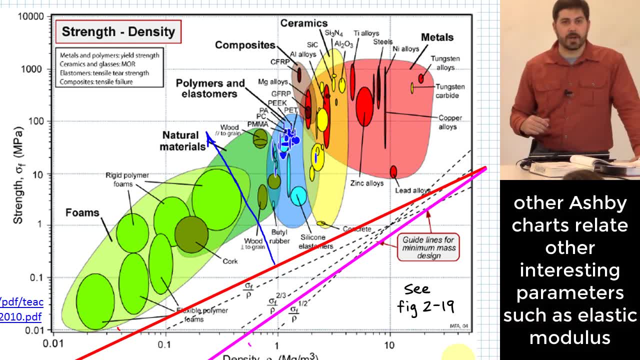 So that's what we're talking about with that particular entry on a chart like this. All right, You can do this for other parameters as well, right? What if you weren't really worried about how much how strong it was? What if you're worried about how much it deforms, right? 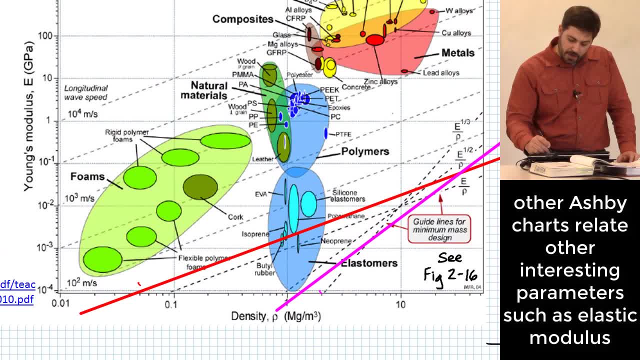 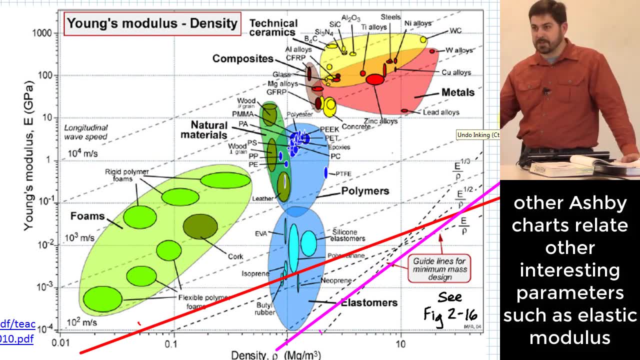 Well, I won't kind of do that one out, But there's another chart that is, you know, relevant to that, And it's one where you're comparing your elastic modulus against the density. So if you're trying to make something that's stiffer and lighter, then you would look at a chart something like this: right, 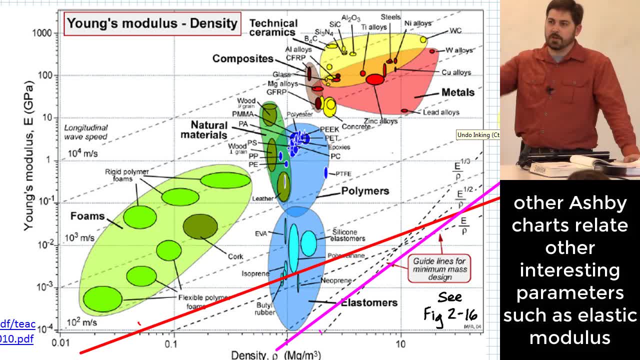 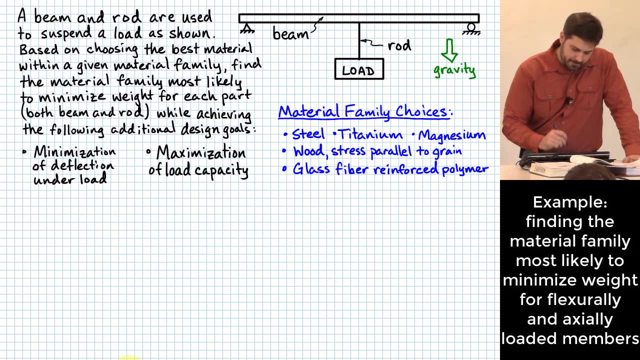 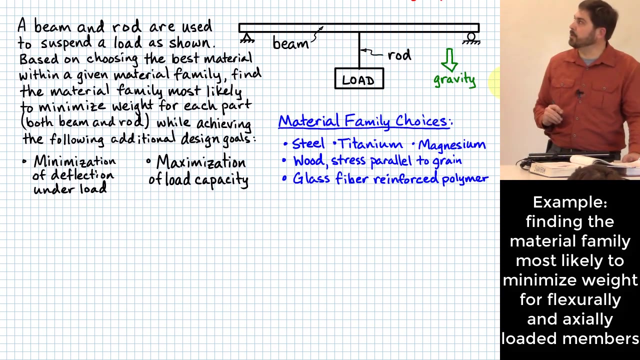 And you could still come up with the guidelines that would help you know what your best entry would be for those cases. Is that interesting? These are called Ashby charts. All right, Let's do a quick example. Okay, Here we have a beam and a rod that are used to suspend a load, like I'm showing here. 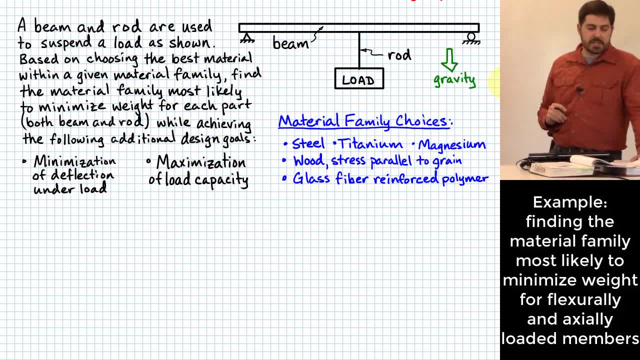 And let's say that we're going to choose the best representative material within each material family. Okay, When I say that I'm talking about some- not the big big material families like composites or metals, I'm talking about a little bit more specific, like metal. 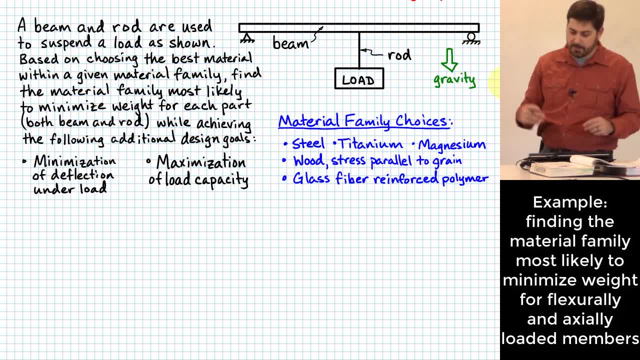 Maybe a family of steels or a family of titanium or a family of magnesium, Those kinds of things, And so, based on choosing the best representative example within each one of those families, find the family that is most likely to minimize our weight for each of the parts: the beam and the rod that's carrying the load. 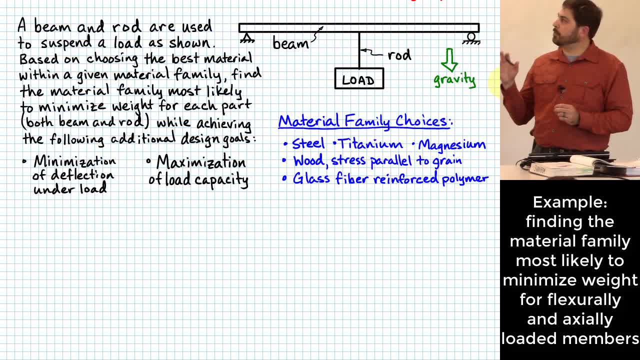 Okay, While achieving these following additional design goals. The first one is we're trying to minimize the deflection of the rod- Okay. And the second one is we're trying to maximize how much load it can carry. We're trying to choose the best material for those factors where what we're trying to do is minimize weight. 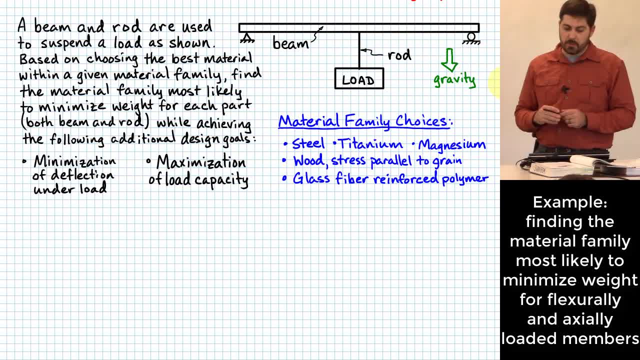 Okay, So let's pick one and get started with it. Which one do you want to do first? Let's start with deflection. But which do you want to do, the beam or the rod, first? Okay, All right, Don't care. 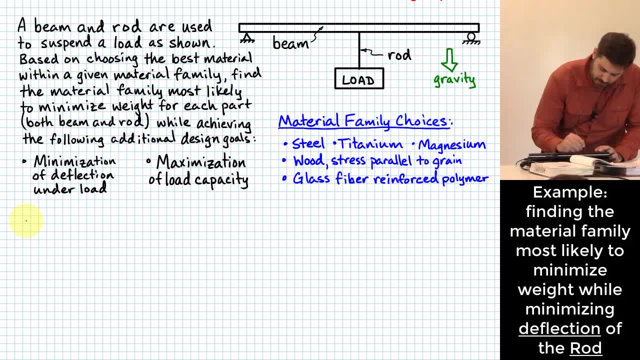 Okay, Let me start with the rod. Okay, And we'll kind of set up a little table here, Okay, So we'll start with the rod. What kind of force does the rod carry? What kind of load does it carry? Axial load. 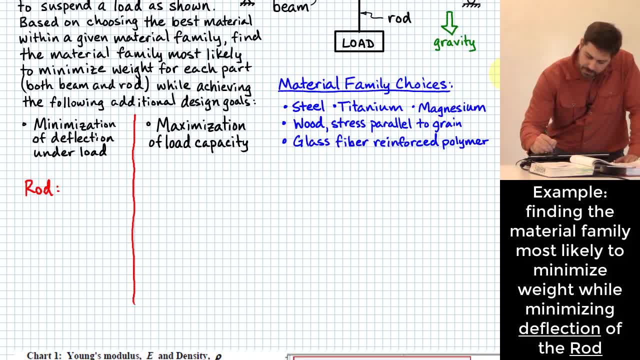 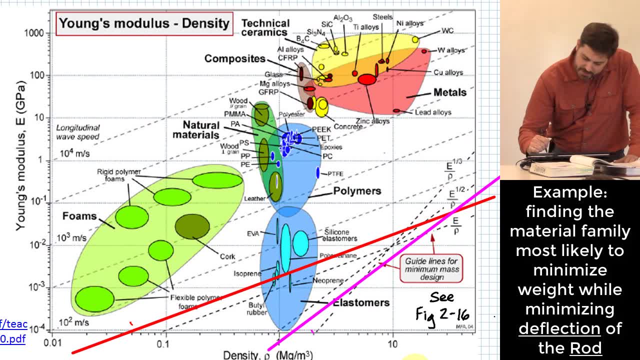 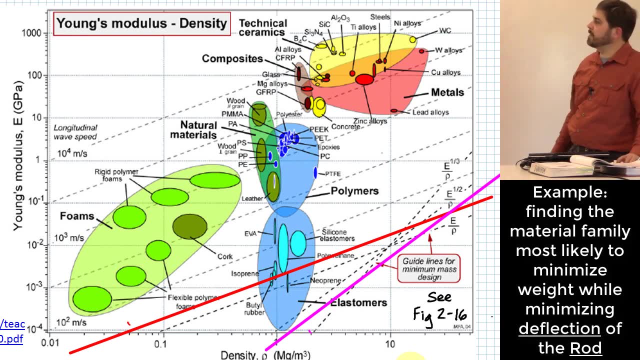 So what do I do if I'm trying to minimize the deflection under load, Okay, While also minimizing weight, Okay. First of all, I have to choose one of my guidelines, All right, And you know, I'll scooch back over here real quick. 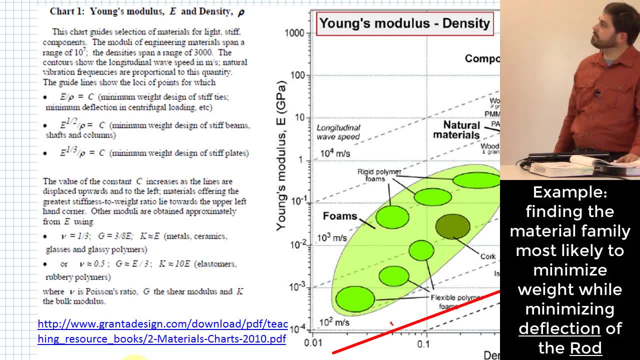 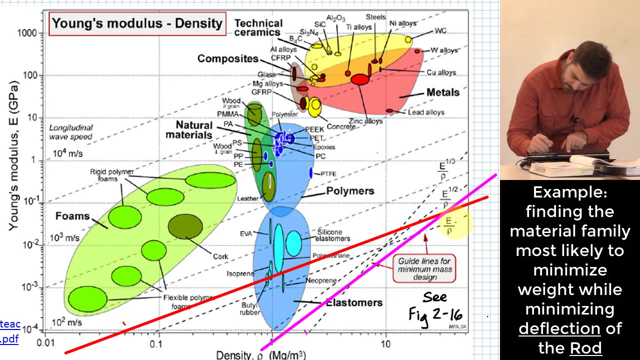 What if I've got? I'm trying to design stiff ties. Which guideline should I use based on this little stuff over here on the left, The one that's just elastic modulus over density? Okay So, elastic modulus over density? that would be this line right here, the red one. 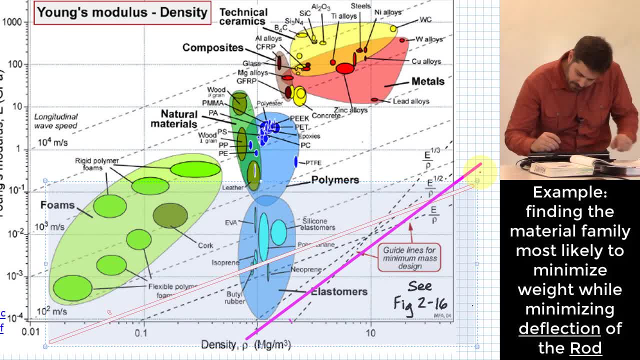 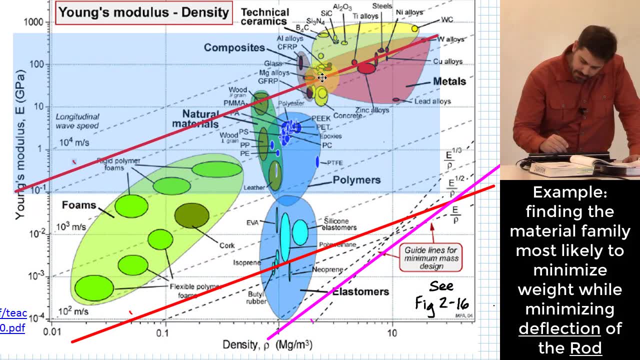 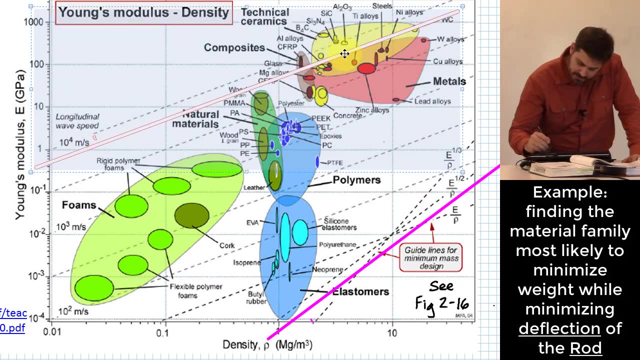 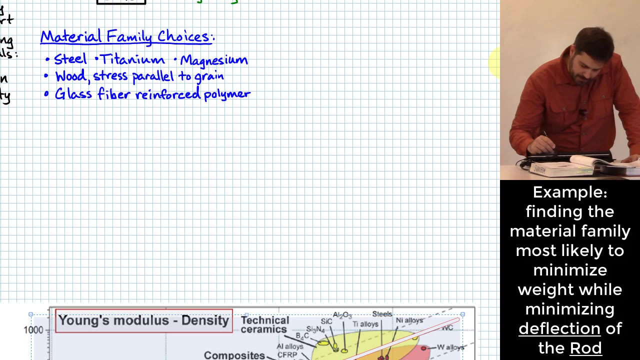 Okay, And so what I can do is take that line and start moving it up Right Until I get out as far as I possibly can within my possibilities that I had in my initial list. What were those possibilities? Steel, titanium, magnesium, wood stress parallel to the grain, glass fiber, reinforced polymer. 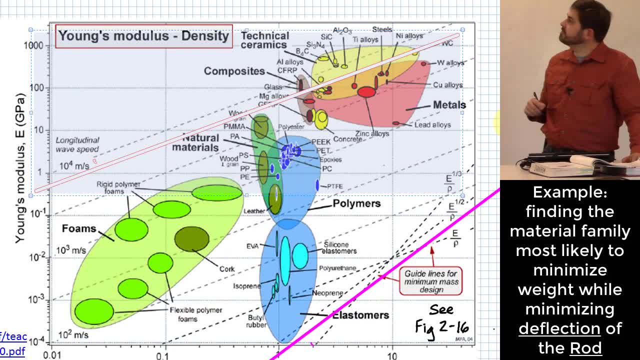 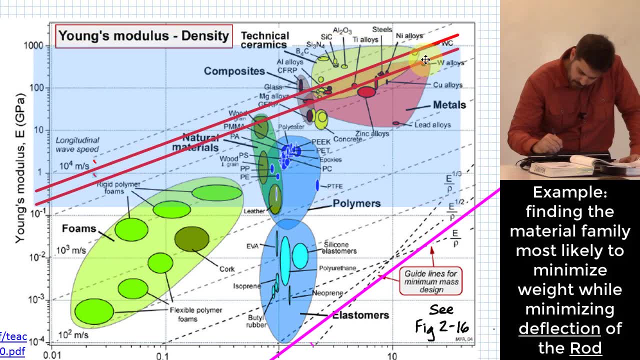 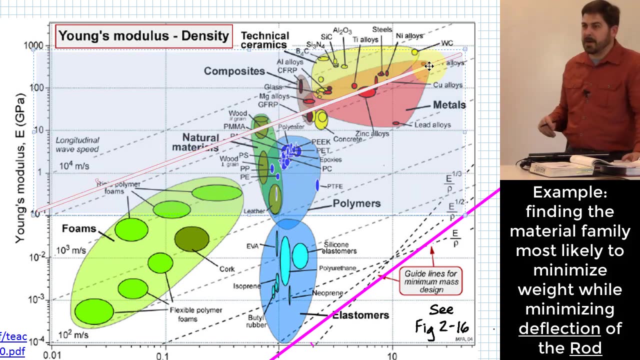 So what's my best choice? Okay, Where's glass fiber? here's glass fiber, reinforced polymer. If I, if that's my best choice, I can basically set that line tangent to the top edge of the, to the top edge of that little circle, right there. 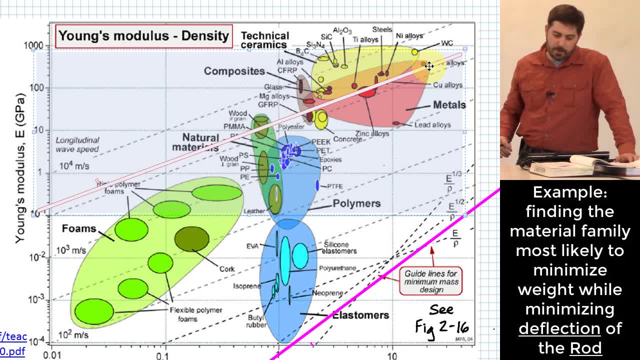 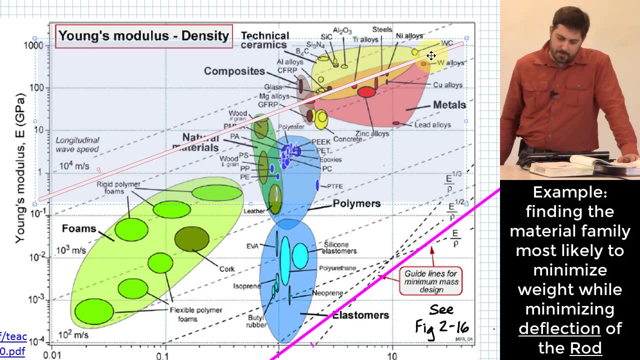 Now look at my other materials. Is what I just came up with better than titanium? Okay, This says titanium alloys right here. No, so I can move it up at least to that edge Right Now. is that better than steels? 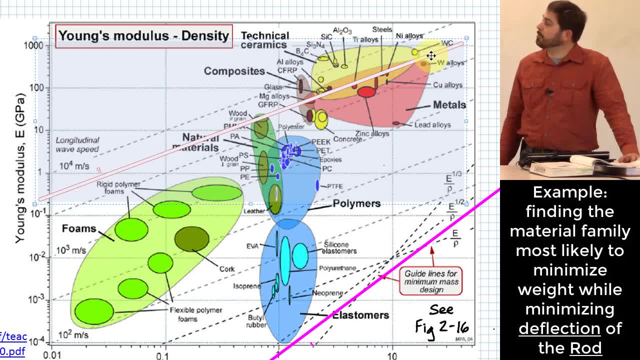 Man, they're pretty close, aren't they? Is it better than aluminum? These are a little hard to say, aren't they? Like? they're all kind of bunched in there. Let's kind of move it up a little bit more. 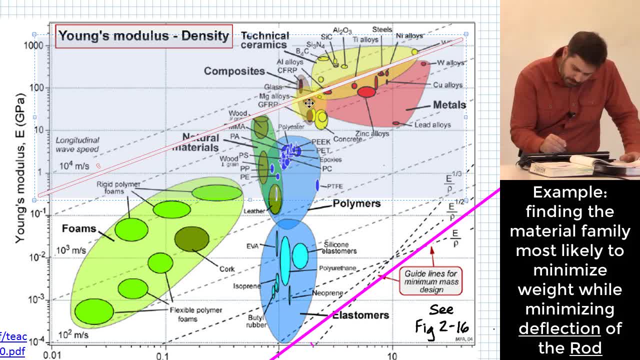 Okay, We got magnesium alloys right here. I've got steels right here. I've got aluminum alloys in that little circle right there, Right, So, based on the ones that I gave you, it might be kind of hard to tell what's the best. 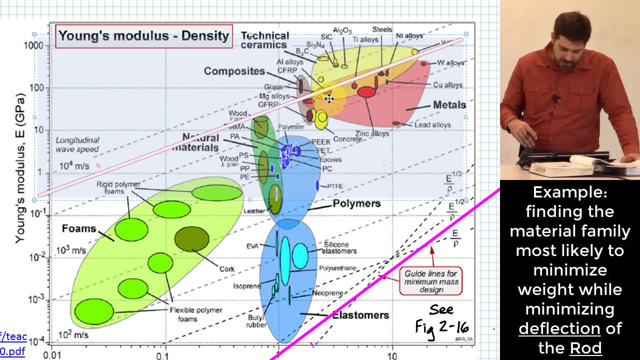 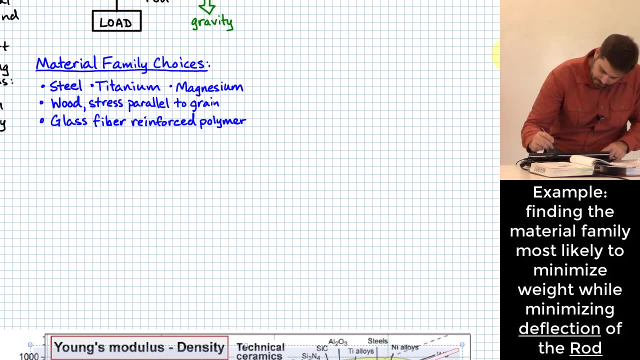 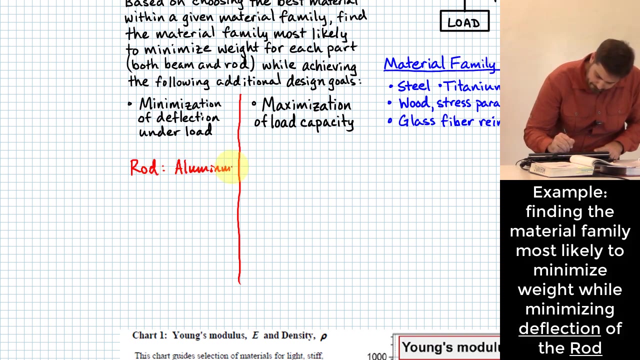 Let's make a judgment call. Okay, Which one looks like? it's the, you know the highest here. Okay, Aluminum looks pretty good, doesn't it? So let's just go ahead and call that. Maybe I'll say aluminum. 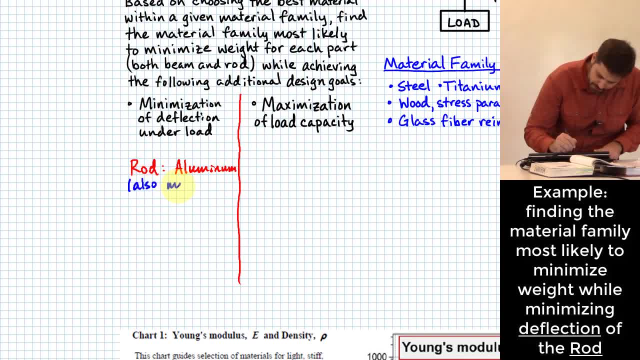 And then maybe I'll put down below: So: maybe steel, Maybe magnesium, Right, It's not. this isn't something that you know. maybe I should have given you a different list to choose amongst Right. That way it would have been a little more obvious which one was the best choice. 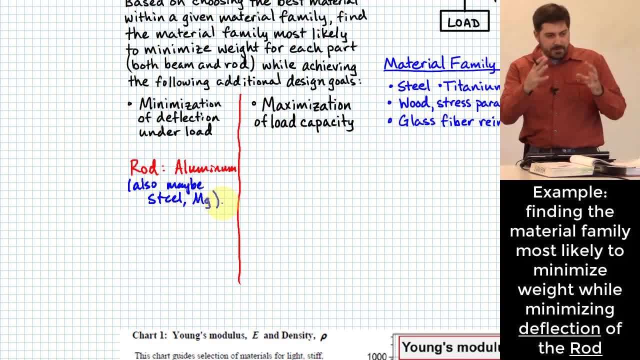 But you can see there. that's why you might see a lot of different choices of different kinds of materials for a particular application. Maybe it doesn't matter very much which one you pick. Maybe you can kind of maximize or minimize the weight using several different kinds and get pretty close, regardless of which one you choose. 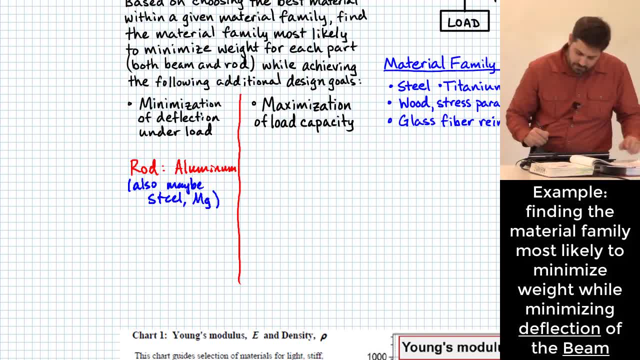 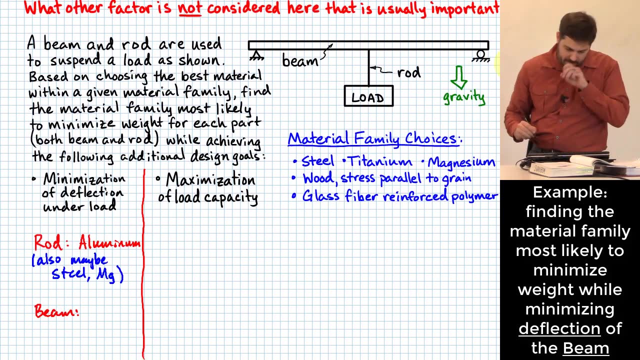 Okay, Which one do you want to do next? Okay, How about we do the beam? All right, We're still trying to minimize the deflection under load. Okay, What kind of load is the beam carrying? Flexural Right. 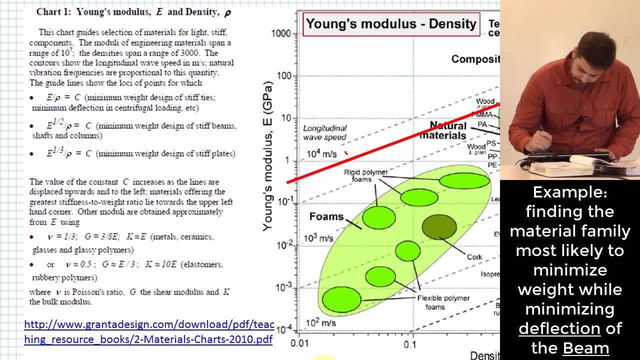 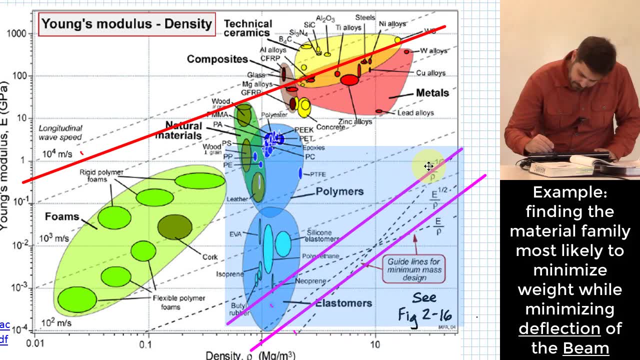 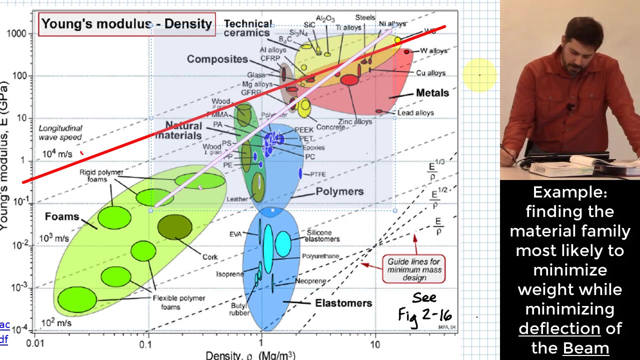 So when I go down into my chart down here, instead of picking the red line, I'm going to pick this little pink line right here. Okay, Now let me check titanium. Okay, Is titanium better than steel? Okay, Is it the best one? 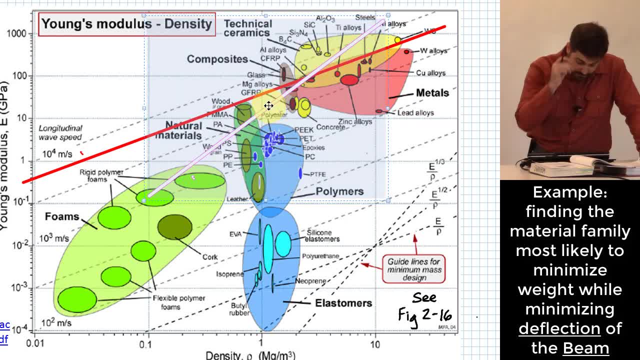 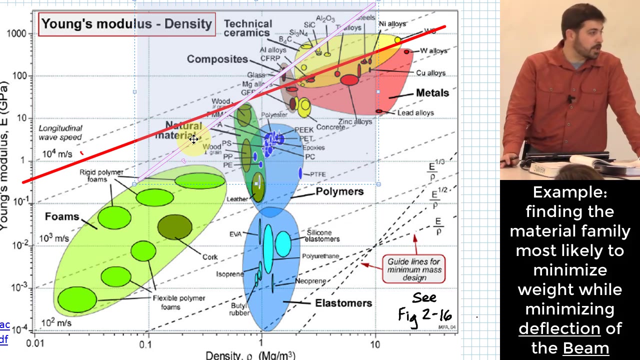 Okay, Here's aluminum. Is that our best one? What's a better one than that? Okay, There's magnesium there. Is there anything better than that? Yeah, Check this out: Wood parallel to the grain. Okay, Turns out that's a pretty good representative type of material to be able to carry flexural stress. 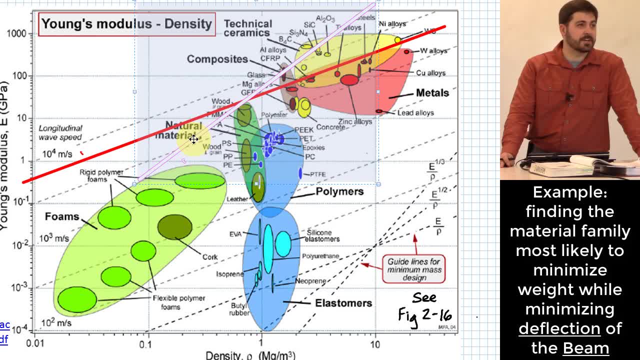 Kind of interesting. huh Yeah, Are you designing what's better for that line? Okay, The further I can move this line up- you know the perpendicular to the direction that the line goes right- the further up I can move it, the better I've got. 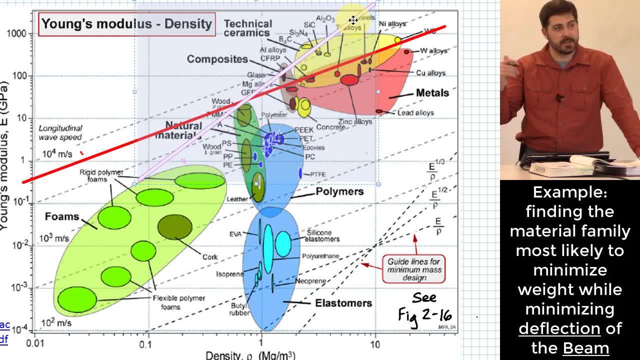 Like that's a better material at carrying that kind of load, the further up I can move it, Right, And so what I'm doing is I'm looking within each of these lines, Right, And so what I'm doing is I'm looking within. each one of these little circles represents a family of materials. 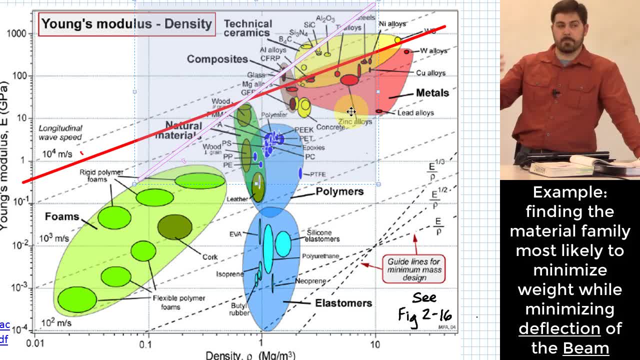 And I'm going to basically make this comparison based on the best representative with each one of those families. So I'm kind of taking it up to where it's tangent with those circles And that would be kind of the best option that I would have for any one of those families of materials. 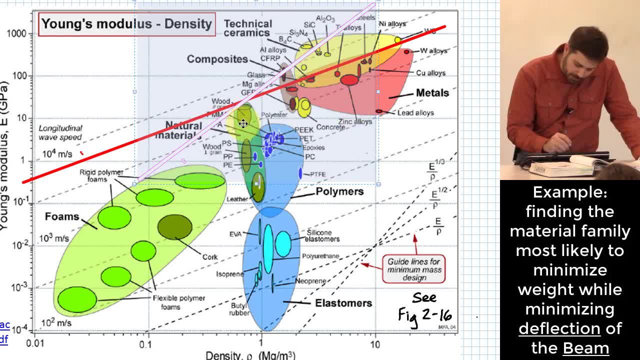 Does that make sense? So where I move this up? I brought it up to where it says here: wood parallel with the grain. That would be this little circle right here it looks like, And so I'm taking it to where it's approximately tangent with that little circle. 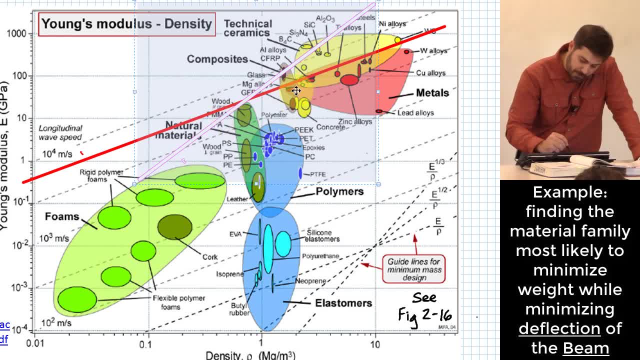 Right, And you can see there that then the line goes above magnesium alloys. It goes above titanium alloys because of the slope of it. It's saying you have a better chance of maximizing this for wood than for magnesium. Make sense? Okay, All right. 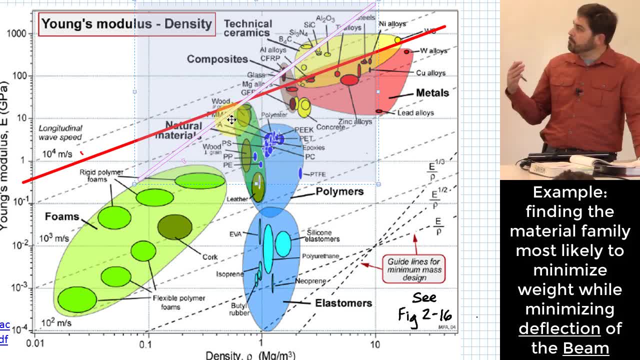 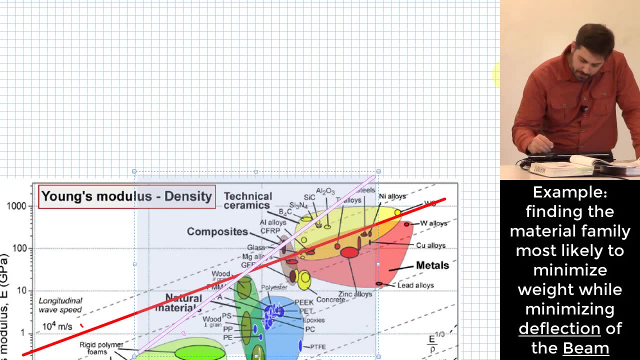 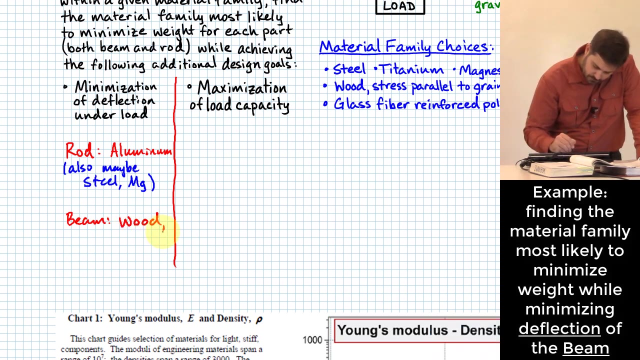 So that, you know, is a minimum mass design for being able to have the smallest amount of deformation, deflection, right for both of the pieces. So we would probably pick wood for the beam and we might pick aluminum for the rod. 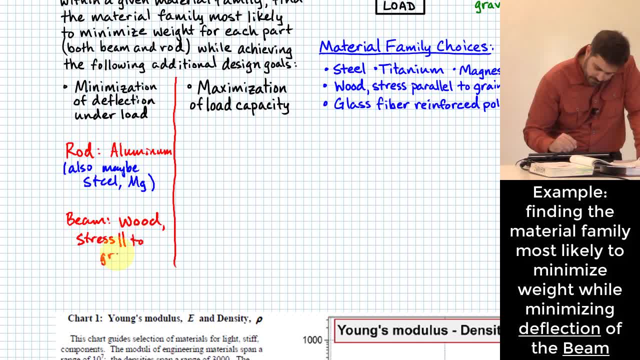 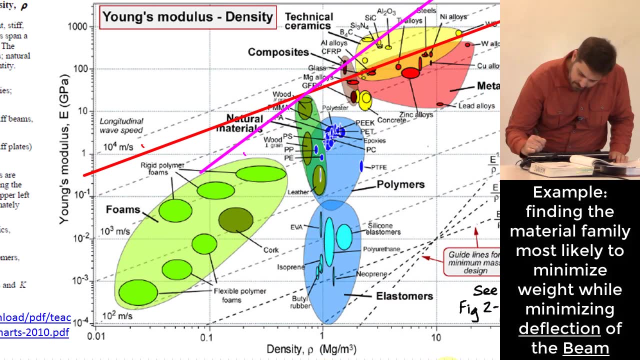 Stress parallel to grain, And that makes a difference, right? If you have wood and you put the stress perpendicular to the grain, what does that do? That's actually on here also, by the way. Where is it on here? Wood perpendicular to the grain- is this circle right here? 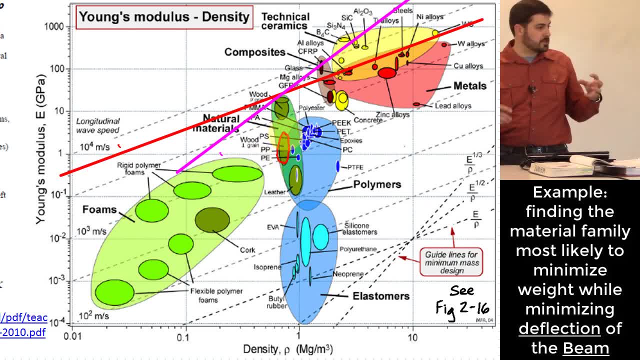 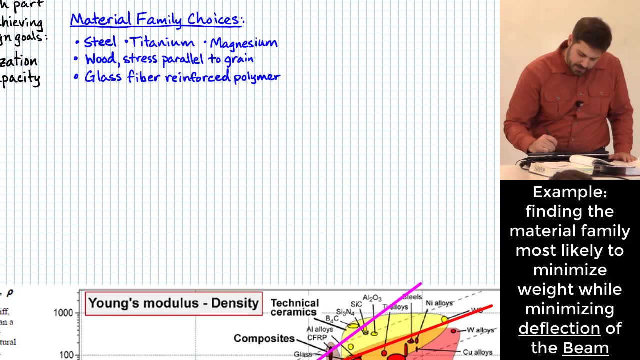 Right, It's less strong, if you're going to try to stress it. so, where you're pulling the grain apart as opposed to pulling along the direction of the grain- Okay, Interesting, huh. What about the next part, where what we're going to try to do is maximize the load capacity while minimizing weight? 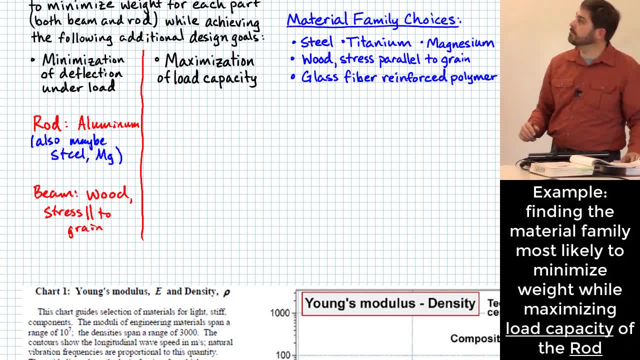 Okay, And we'll do that for the rod. What matters for this? This is the one we initially looked at. What matters for this? This is the one we initially looked at. Okay, This is the one we initially looked at, right. 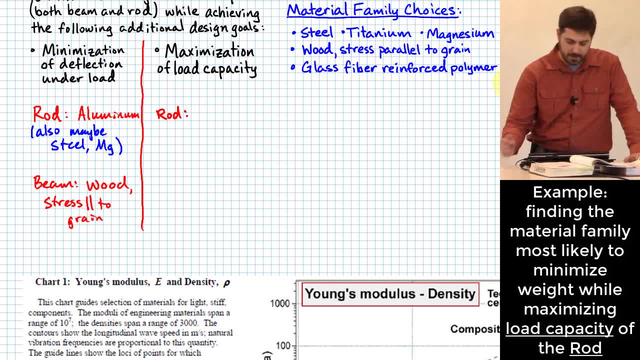 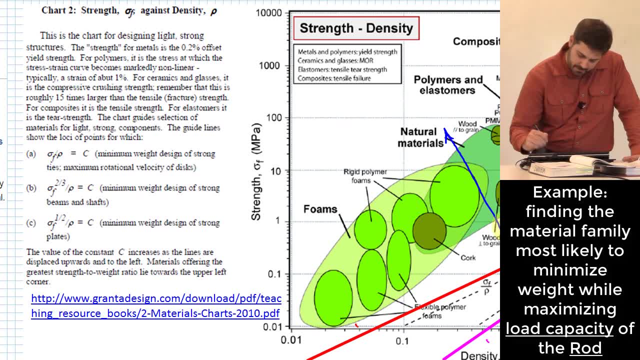 This is the strength. We have to compare strength versus weight in order to determine this question of maximizing your load capacity per weight. So we go down here to our other chart and we say for the rod we'll pick the line that represents axial loading. 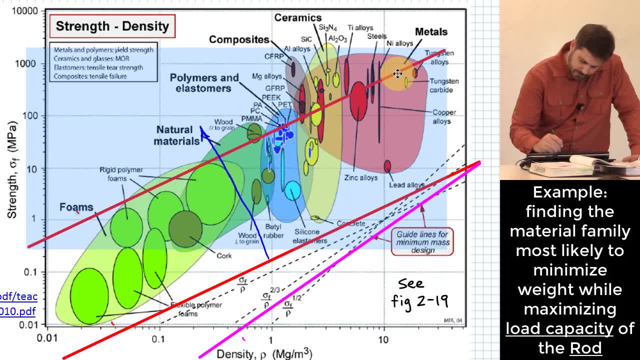 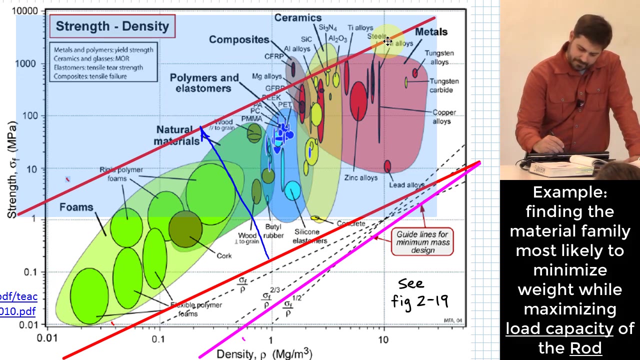 Right, We'll try to move it up here. Okay, Here's wood parallel to the grain. Is there anything better than that? Titanium is better. Anything better than that. I mean there are some things better, but anything that was in the list that I gave you to pick between. 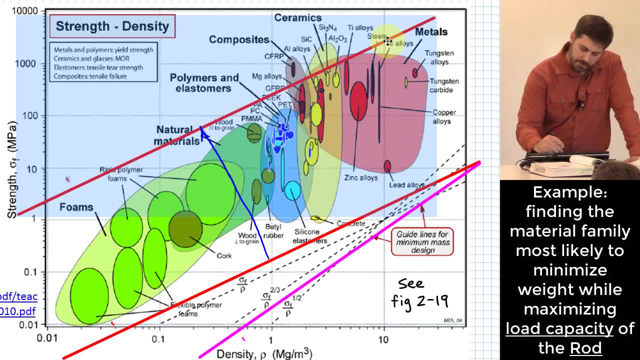 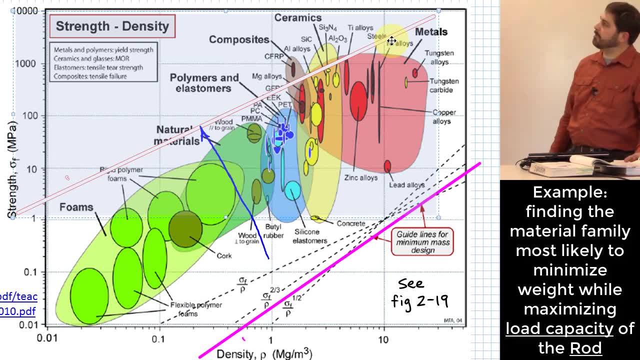 Okay, Looks like that might be a pretty good choice, with one possible, you know kind of possibility there. Which one? Okay, Look for aluminum, Look for aluminum. there, Aluminum is pretty close. What about magnesium? All right, Magnesium ends up being pretty close, which, by the way, you don't use pure magnesium. 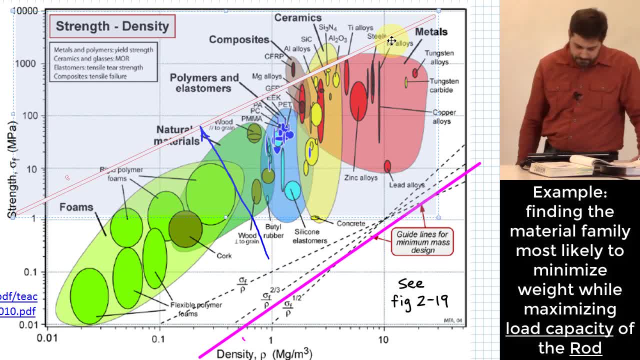 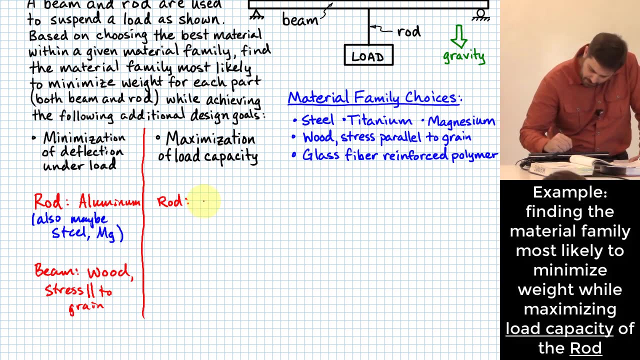 They are magnesium alloys, but all right. So anyway, I'll say this probably looks like titanium is our best choice. I'll go up here and answer this question. for the rod We'll say we'll have to pick titanium if we're trying to maximize our load capacity. 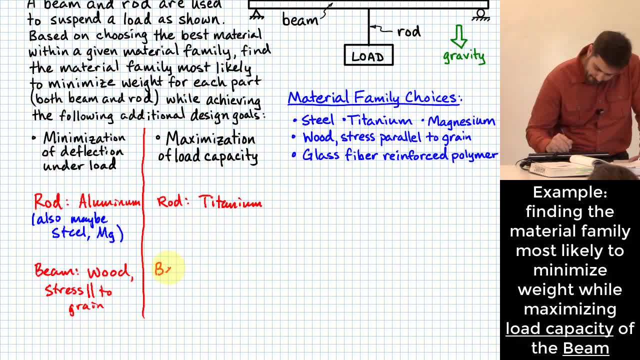 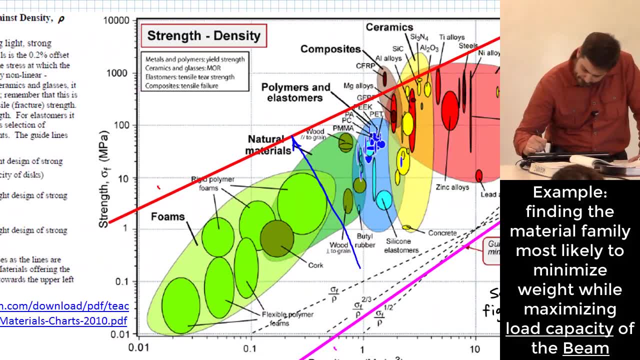 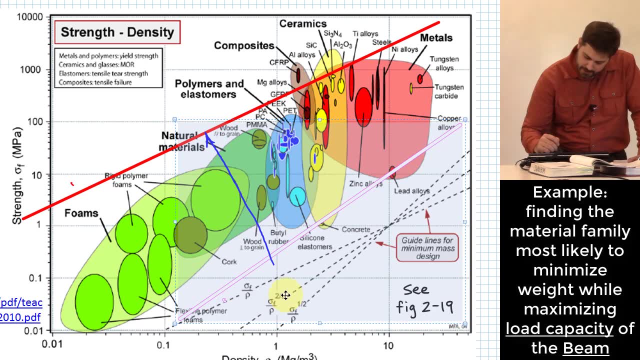 What about the beam? What do we do there? Take this line, which is the one that's appropriate for flexural loading, and move it up. What if I go to? I'll try wood first, Wood parallel to the grain. Is there anything better than that? 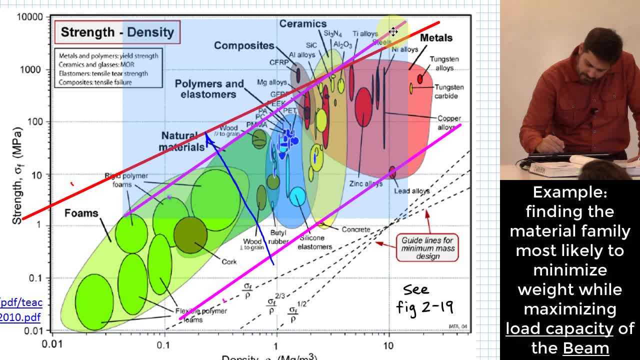 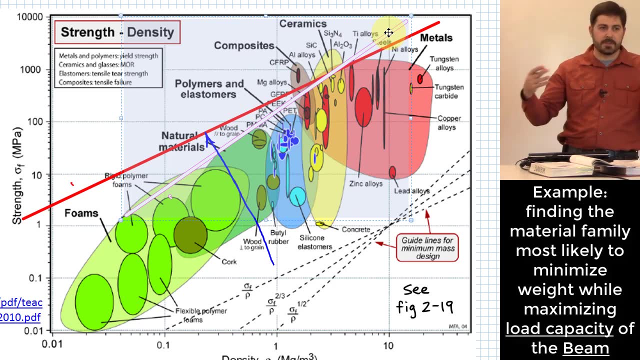 Maybe magnesium by a hair? Okay, That looks like. maybe that would be my best choice of the ones that I gave you the list to check. Right, Maybe not the best overall, but I gave you this list to kind of evaluate these different kinds of materials. 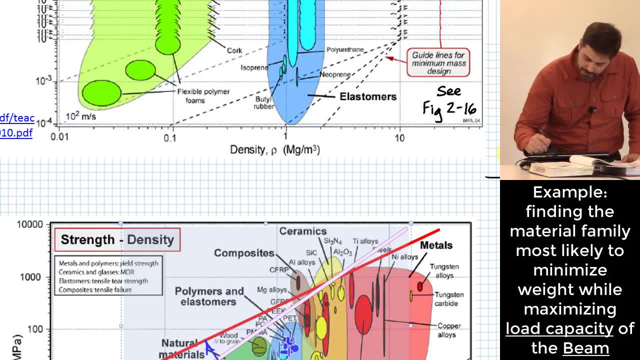 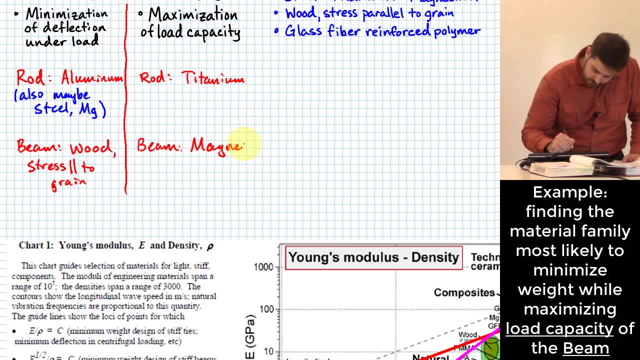 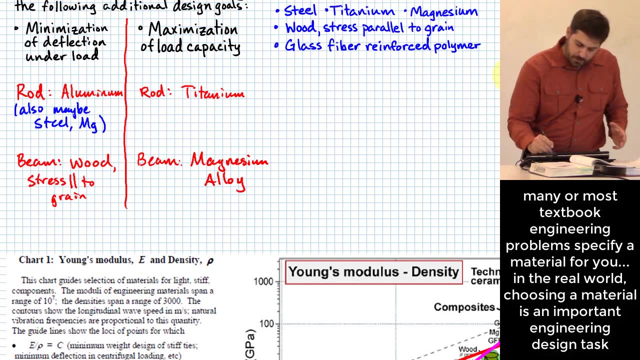 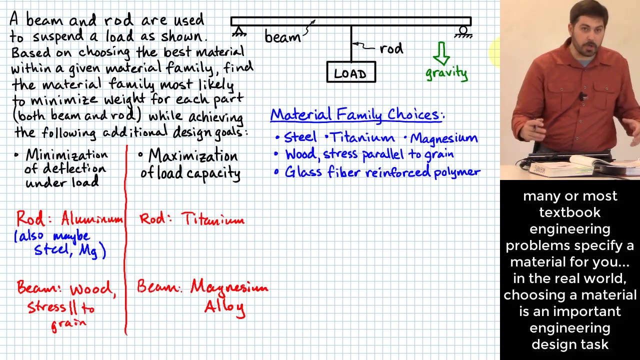 And I would say yeah, And I would say maybe a magnesium alloy in this case. All right, We're not going to do that much throughout the course of this course with this kind of information, But this is kind of the beginnings of a design book, right? 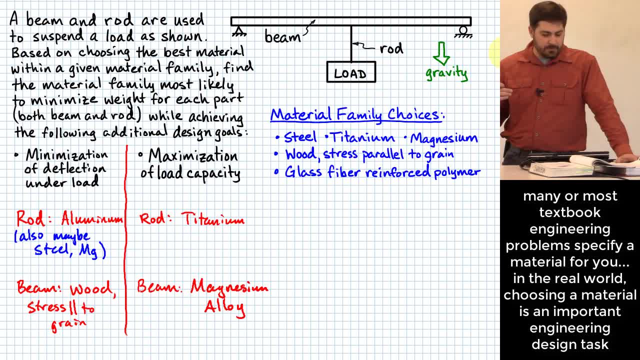 We're trying to learn about how to do mechanical design And for a lot of the exercise problems I give you, I will tell you what kind of material you're going to be using And I won't give you a lot of tasks where you have to decide what kind of material you're going to use. 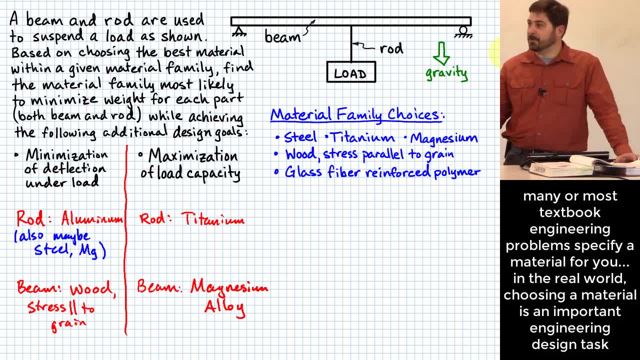 But in the real world, that's something that you would have to probably think about. doing is like I've got to do such and such a task. Do I want to use titanium or do I want to use steel? Do I want to use aluminum? 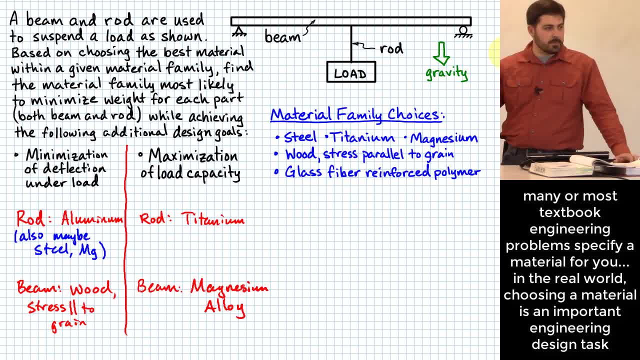 How do I choose Right, And this gives you some level of structure in your mind of thinking about how you might think about. you know what the best material would be to do various kinds of things, What the best material would be to do various kinds of loading. 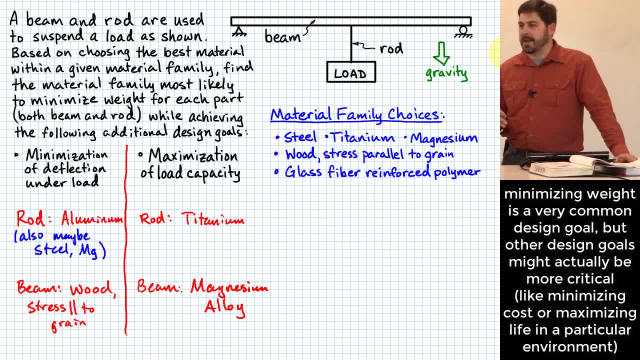 Does that make sense? And being able to reduce weight? Now, I did all of these with respect to the design goal of reducing weight. Is that always the design goal that we're thinking about? No, Okay, As a matter of fact, some of you may have seen this a second ago. 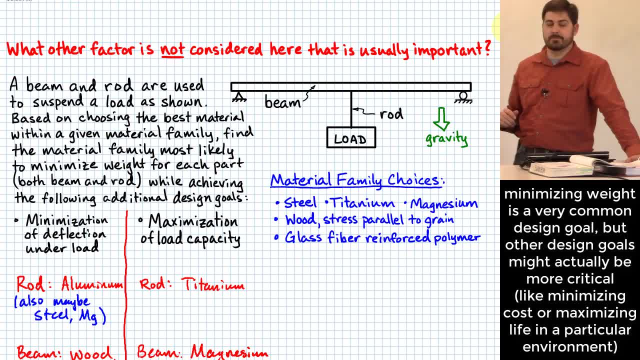 What other factor did we not think about here? that is usually important- Someone mentioned it earlier: Right Cost, Okay, Cost is one of those ones that's almost always important in terms of practical terms. Right, And if you can find a solution to a problem that is less costly and still works, it's very often one that people will want to go with. 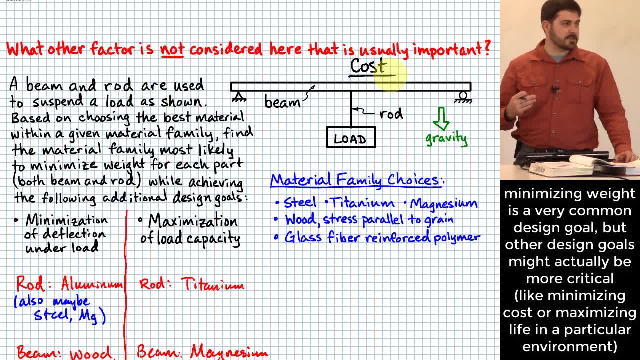 Right, Not always, You know. you think about like road bikes, Right. For some people, cost is not a factor if that's the product that they're trying to, you know trying to, you know, trying to optimize.